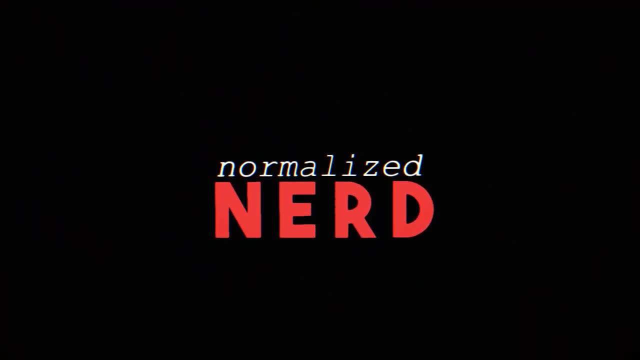 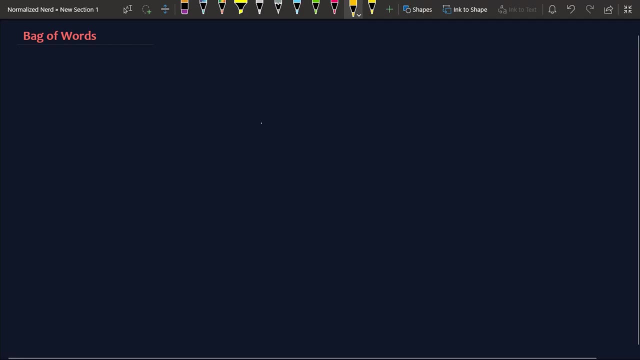 Hello, people from the future, Welcome to Normalize Nerd. So I'm gonna start a new series on NLP- Yes, the Natural Language Processing- and this is the first video of that series, and in this video I'm gonna talk about bag of words model. If you are new to my channel, then please subscribe to my channel and hit the bell icon. I make videos about machine learning and data science regularly. Before starting, 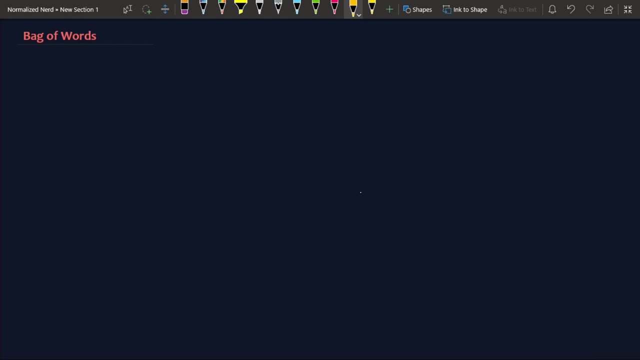 you need to know what is Natural Language Processing and why it is so useful. Well, in simple terms, Natural Language Processing simply means to train a machine learning model which can understand human language- Yes, the language is like Bengali, which is, by the way, my mother tongue- English, Hindi, literally any language that humans speak. there should be a model which is able to understand those things. Now, why it is so important. Well, you can see that there are a lot of 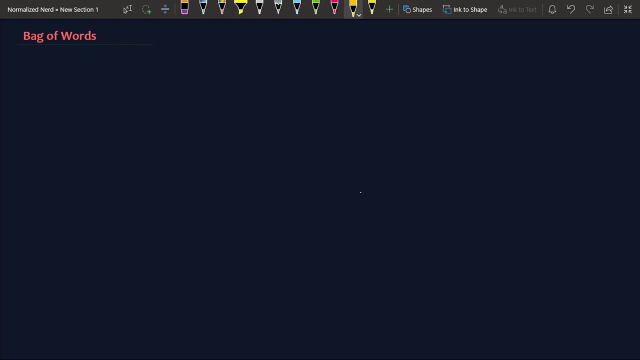 scopes to apply this machine learning models. So there are applications like machine translation, speech to text, text to speech, generating new poems by computers and so on and so forth, But it is notoriously hard to train a machine learning model that can understand human language. Why so? Well, there are actually two reasons, The first one being a machine learning model basically acts on numbers, right. 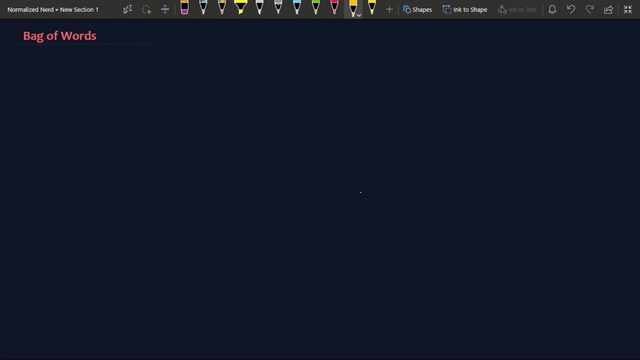 But in human languages there is no numbers involved. Well, if it were the case, then that would be very useful for us, But unfortunately it is not the case. So what we need to do, we need to first convert the natural languages, the human interpreted languages, into numbers, And that is a really hard task to do. And the second one being there are lots and lots of human languages and it is really hard to train a model that can understand every one of them. So 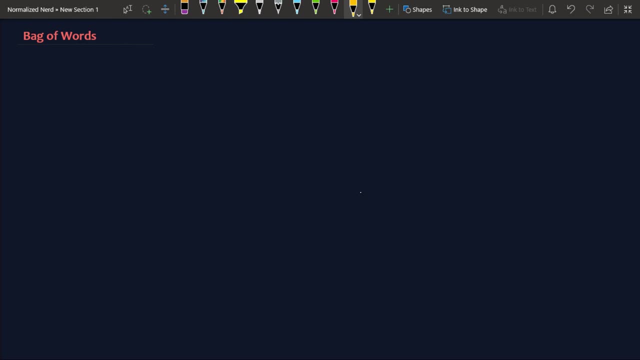 these are the two main reasons why it is very difficult to build a model that can understand human languages. But fortunately, the last decade was a blast for NLP research. We got many useful things. If I want to give you some example, then I should mention Google's BERT, Sequence, Encoder, GRU and, of course, the great what to make models, And the list goes on. But I'm going to stop right here and I'm going to start explaining the concept that I'm going to 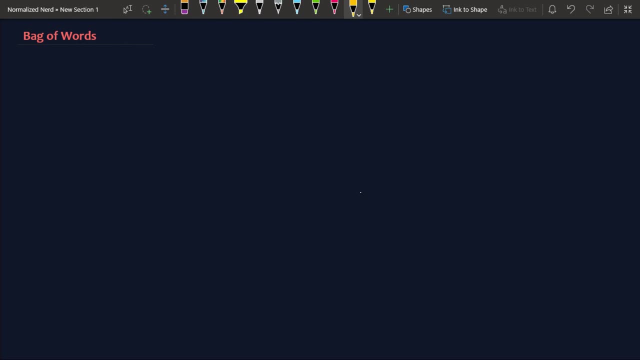 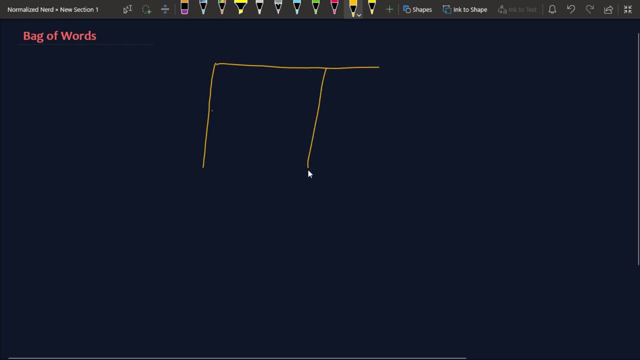 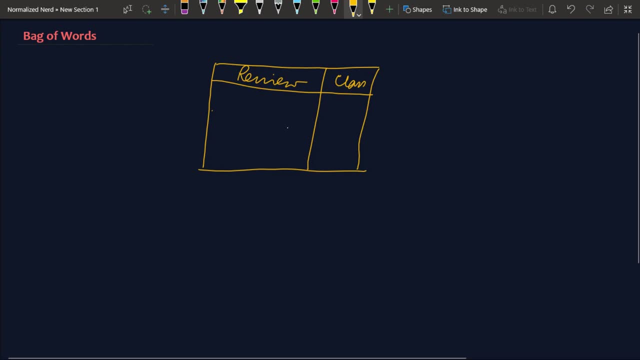 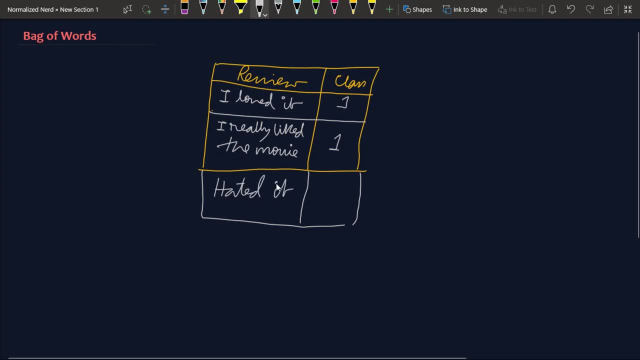 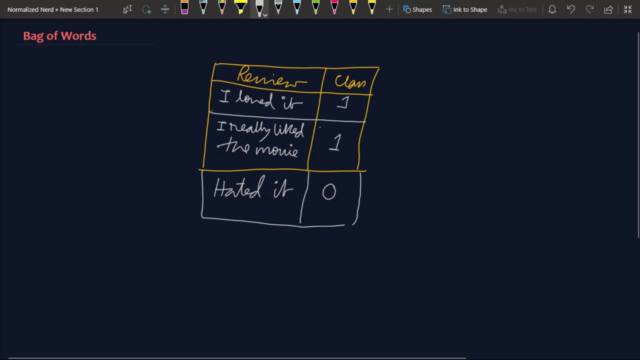 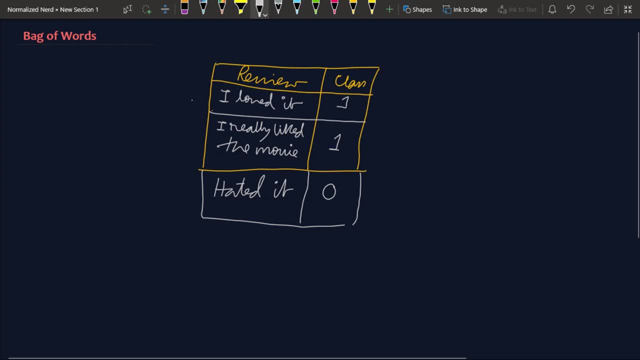 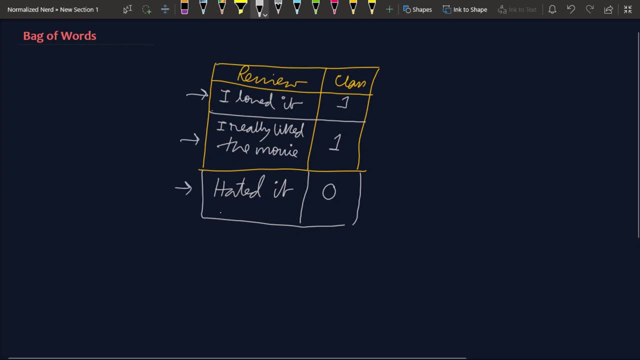 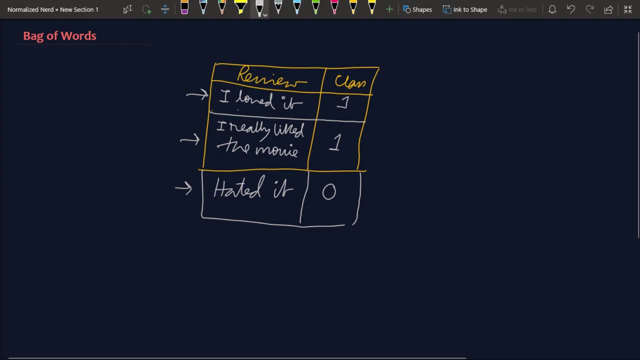 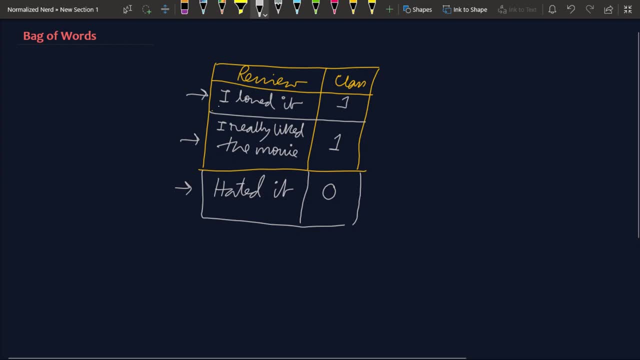 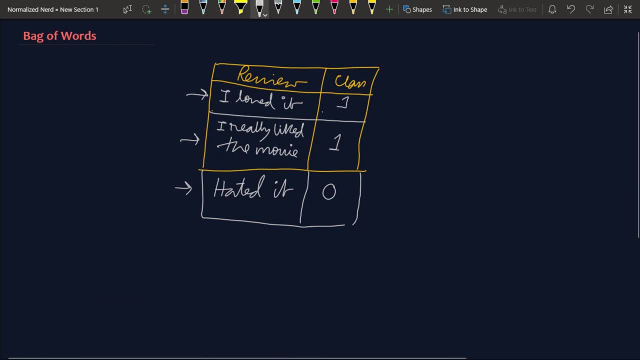 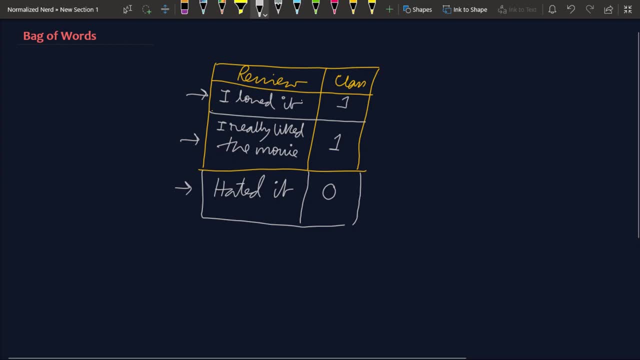 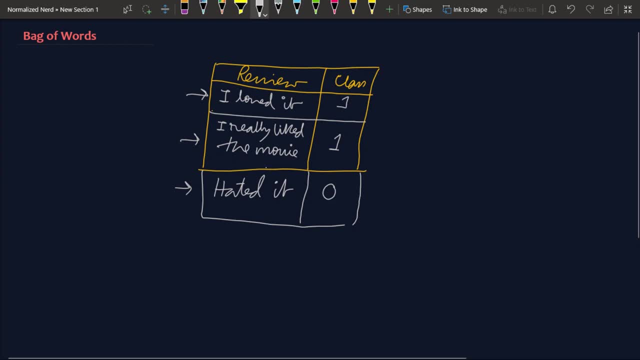 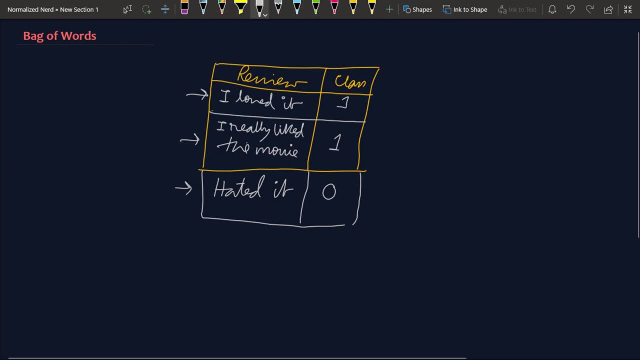 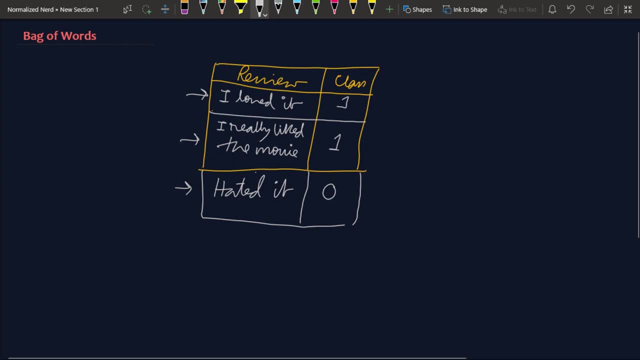 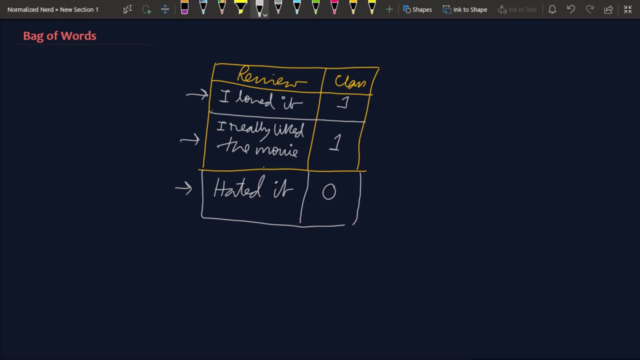 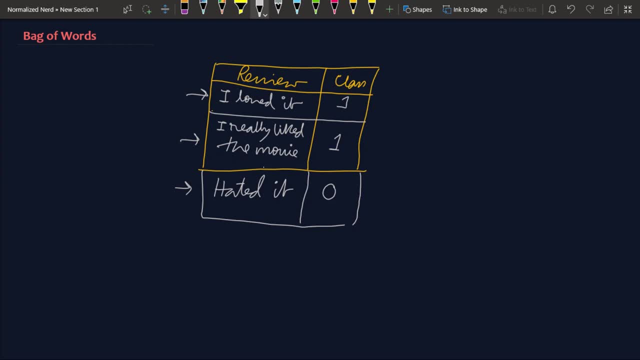 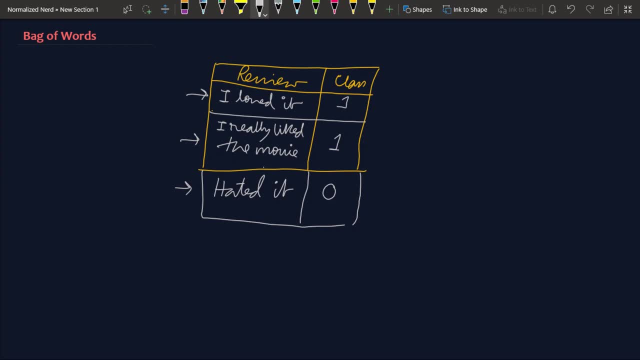 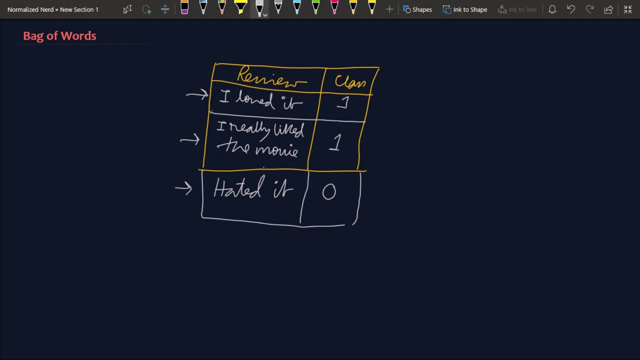 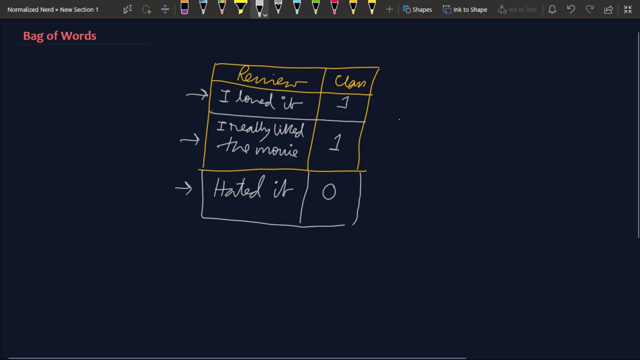 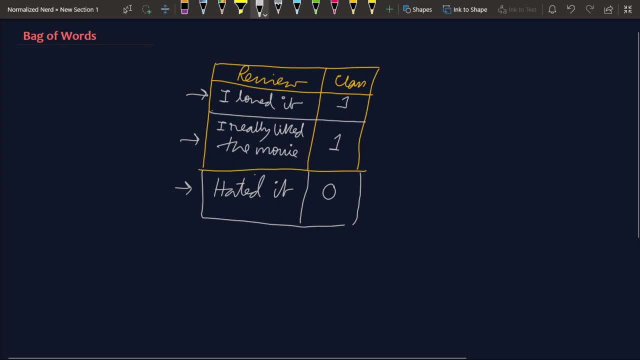 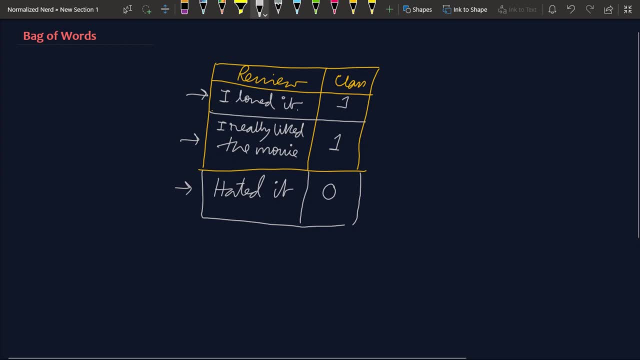 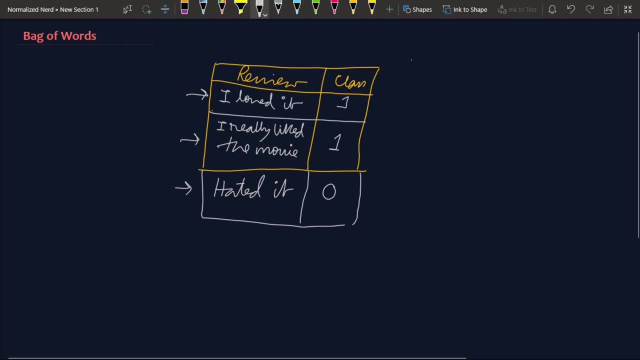 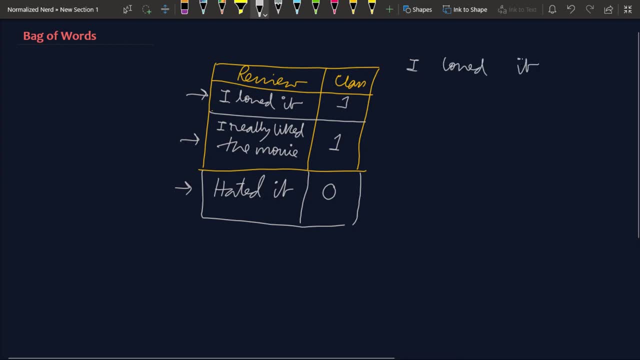 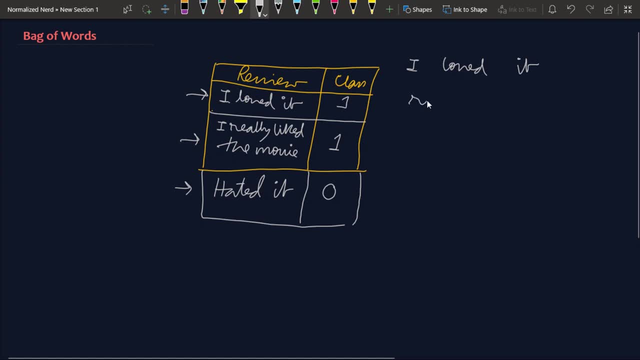 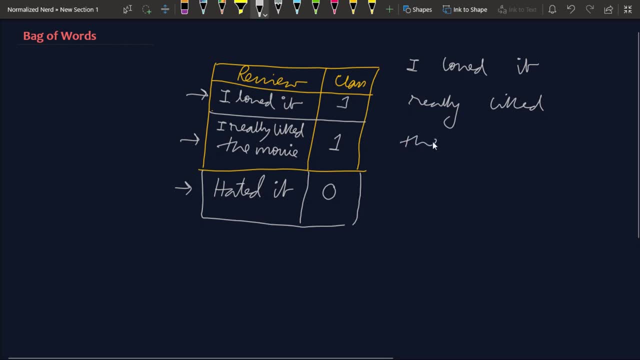 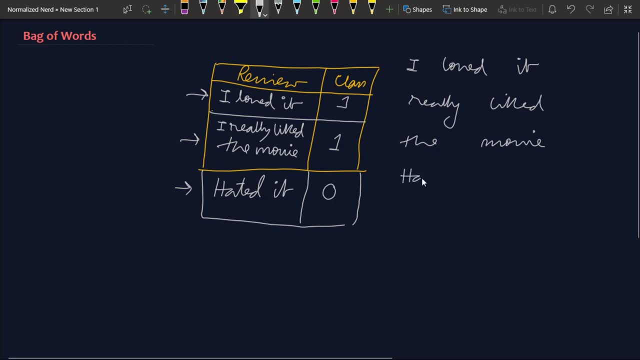 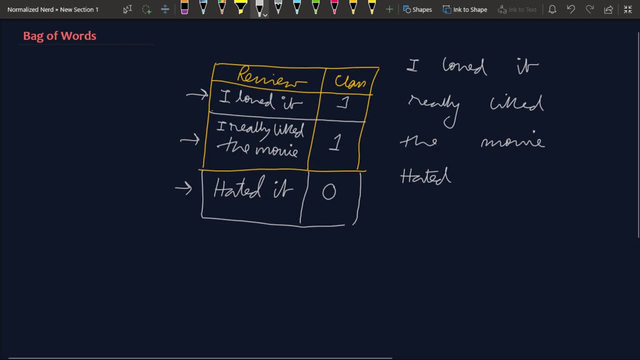 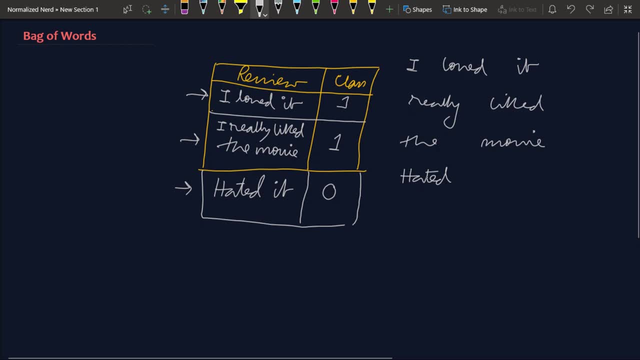 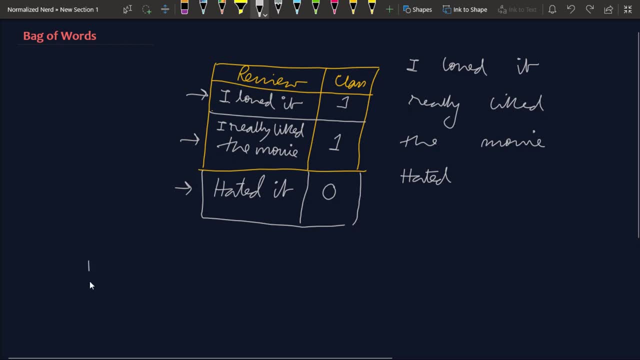 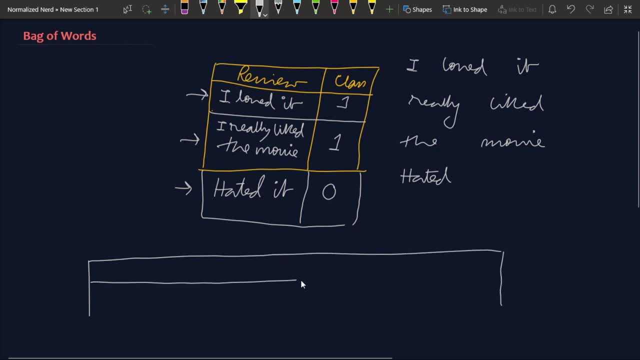 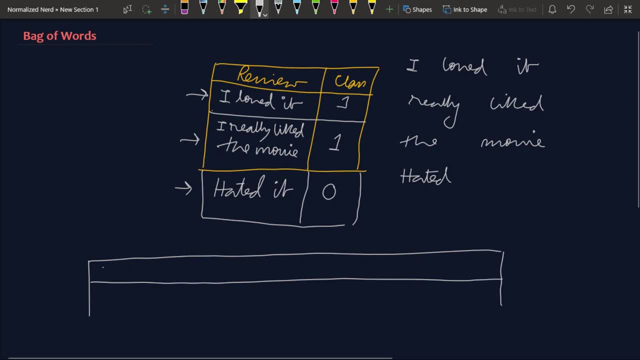 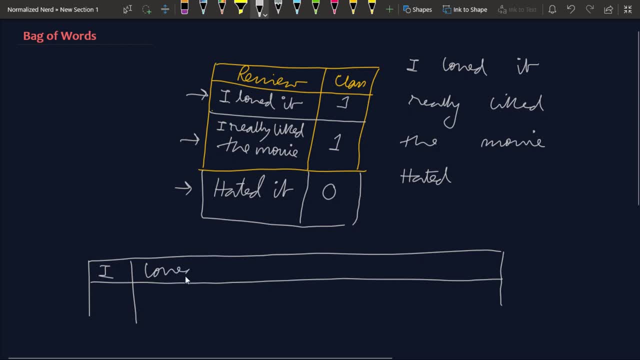 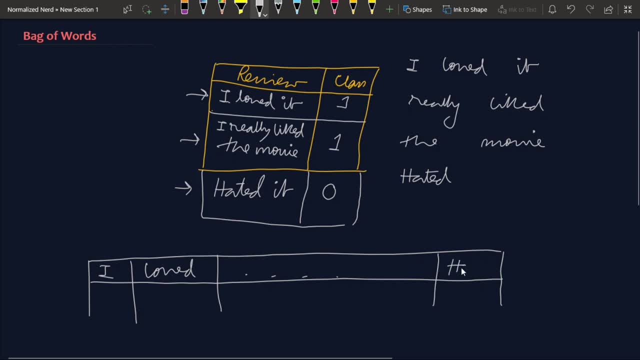 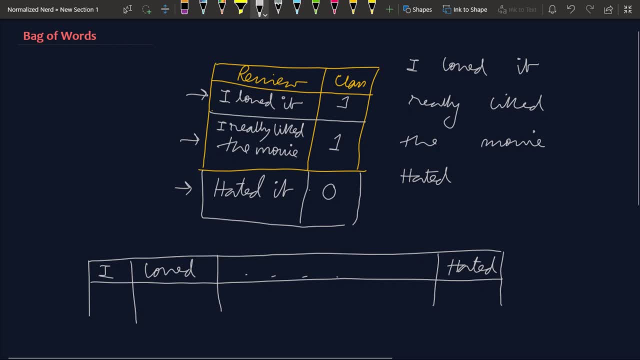 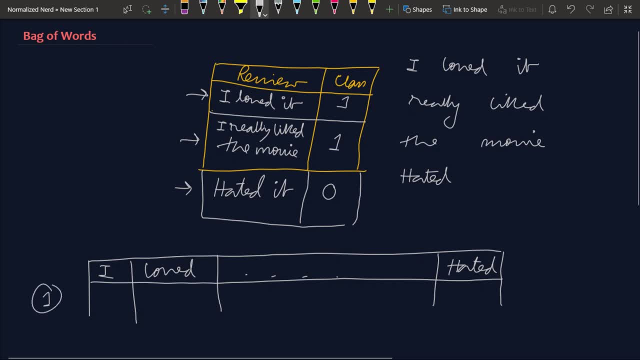 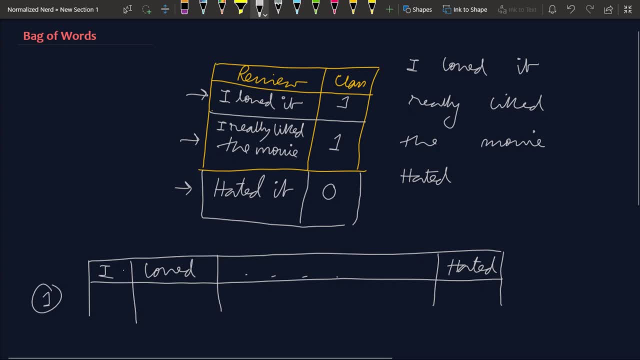 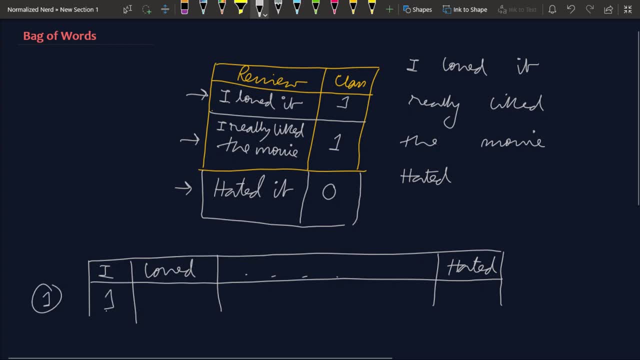 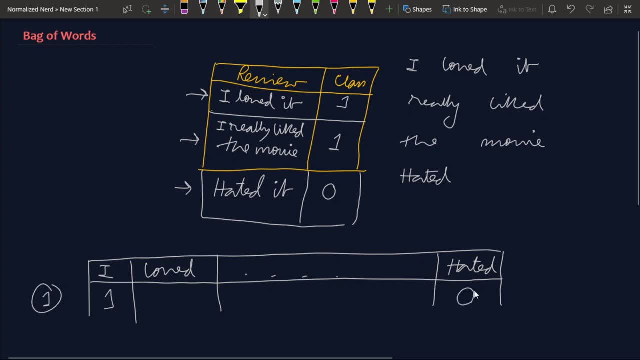 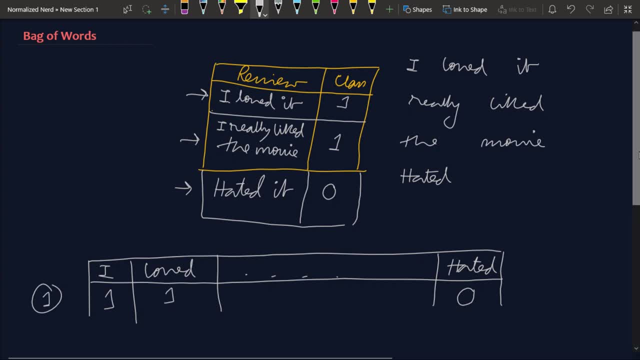 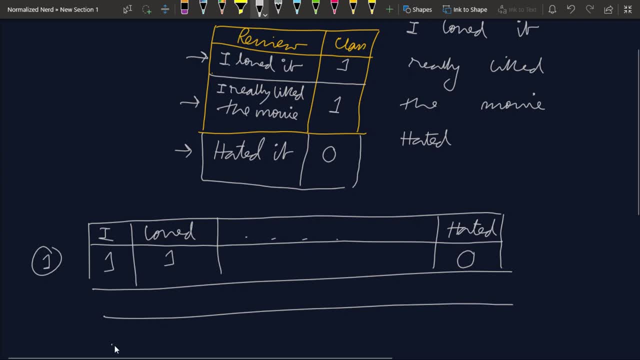 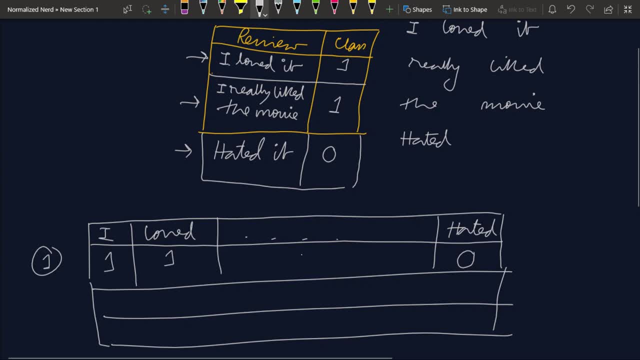 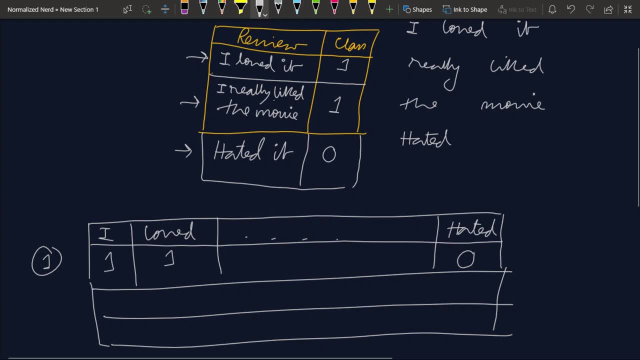 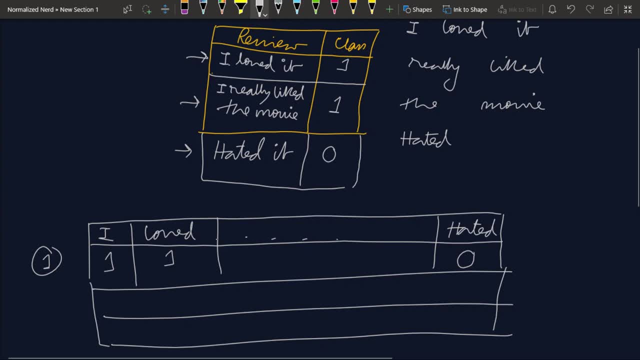 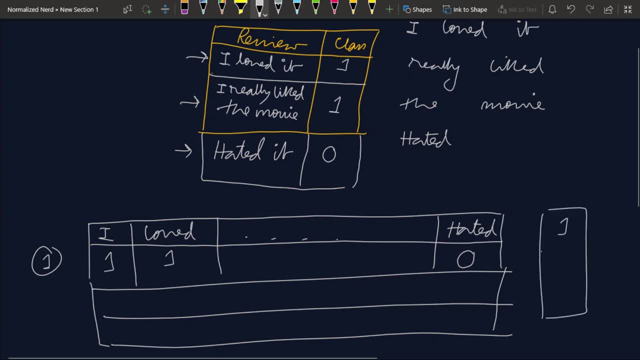 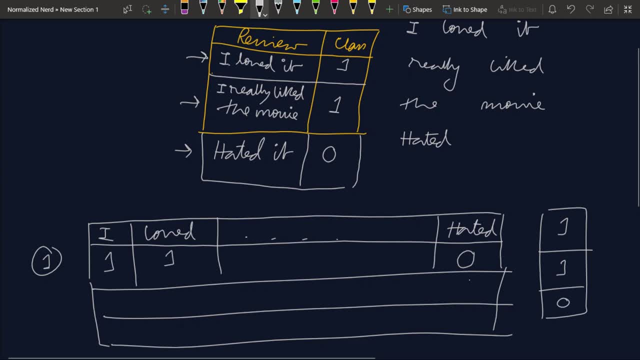 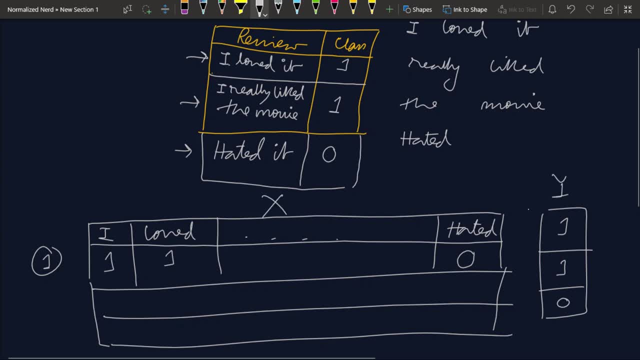 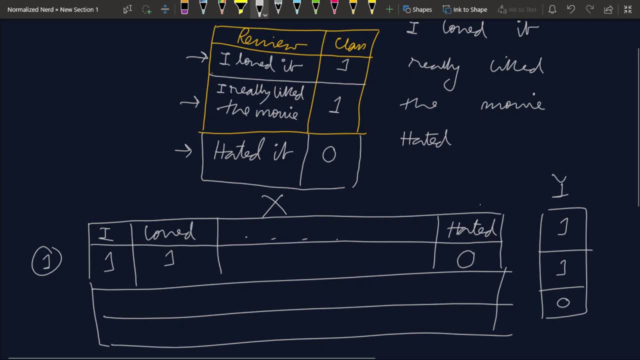 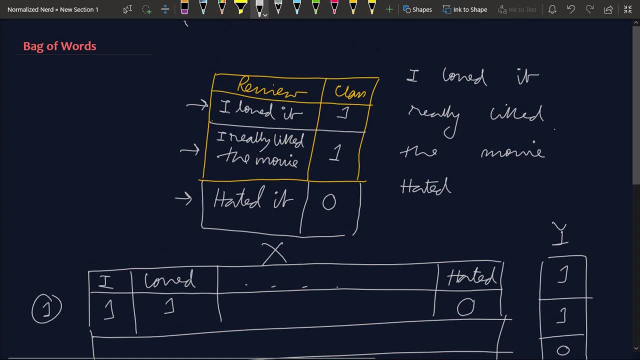 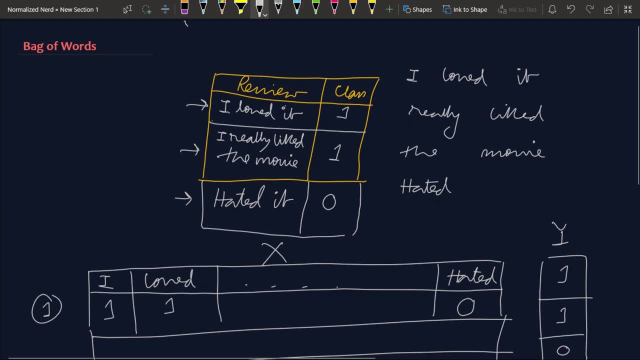 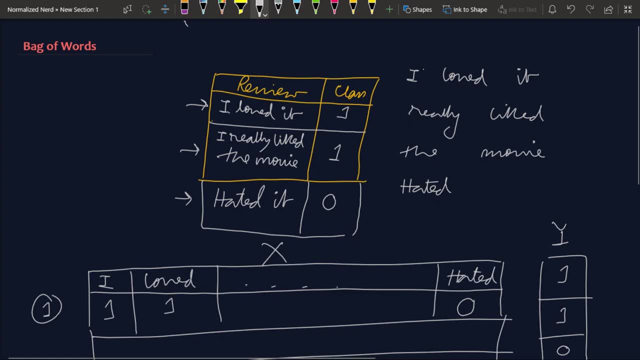 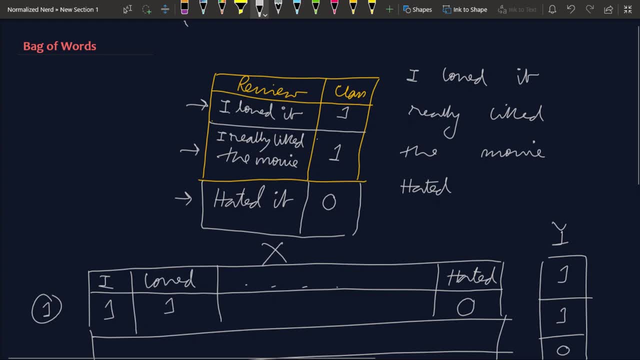 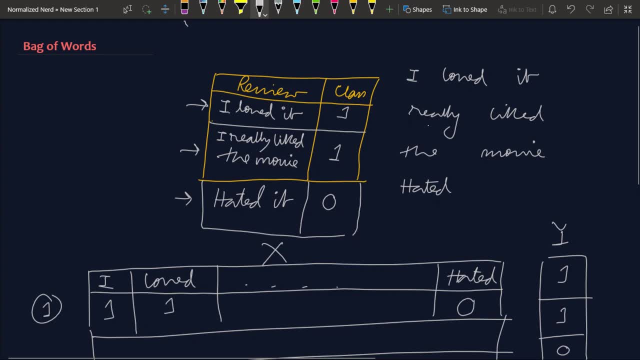 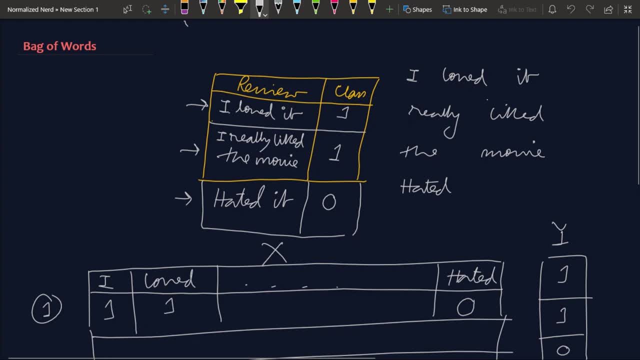 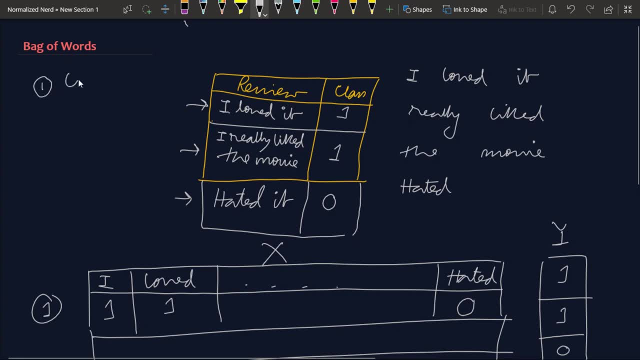 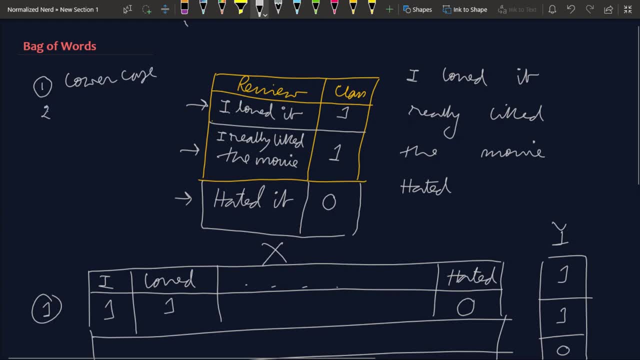 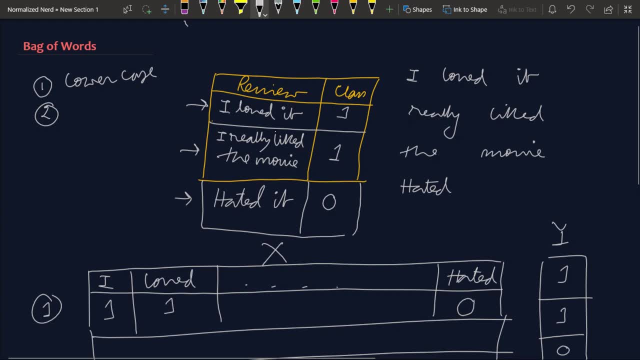 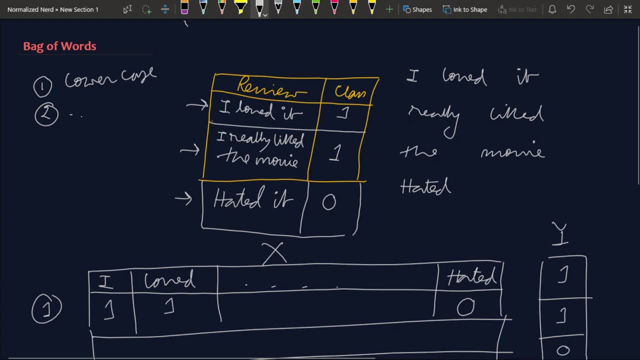 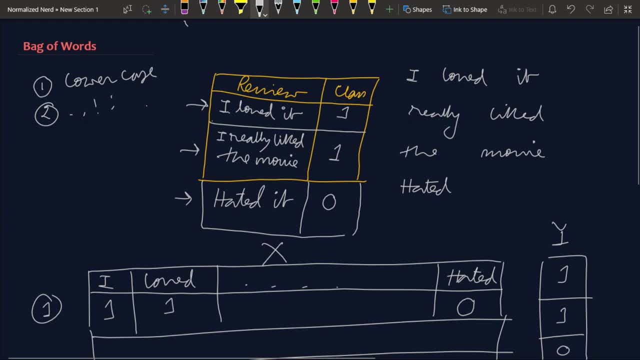 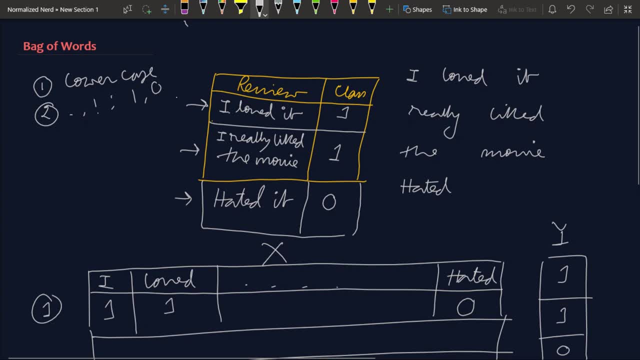 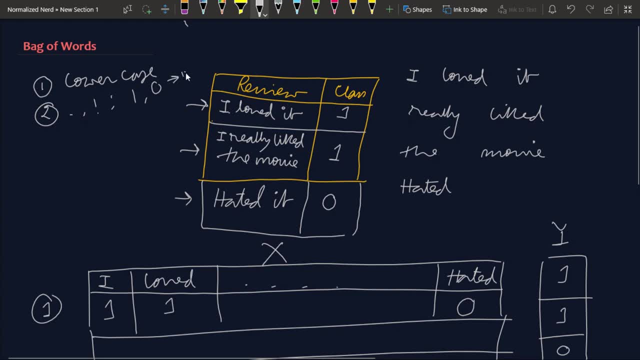 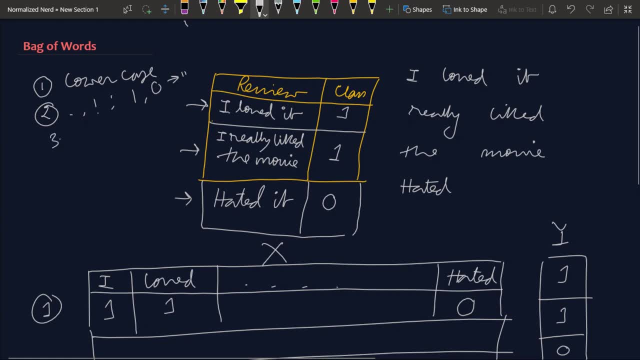 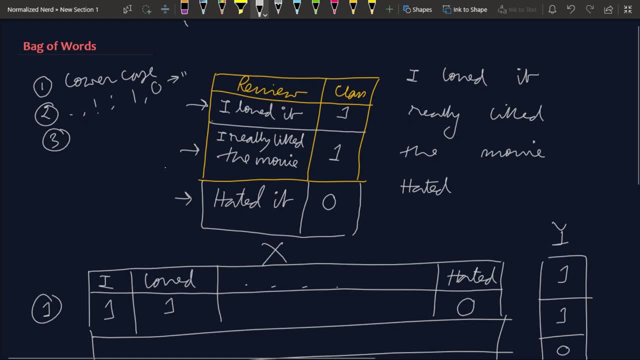 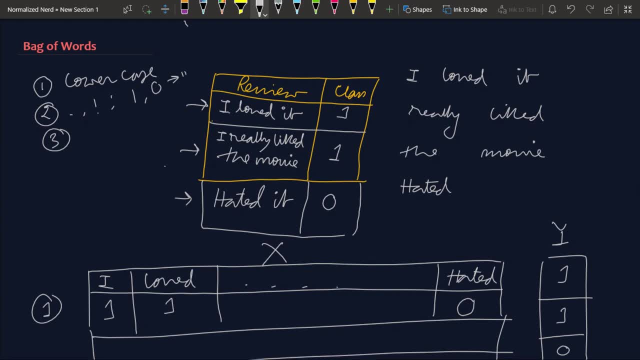 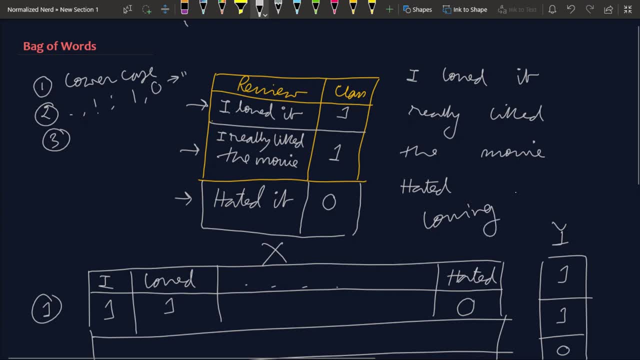 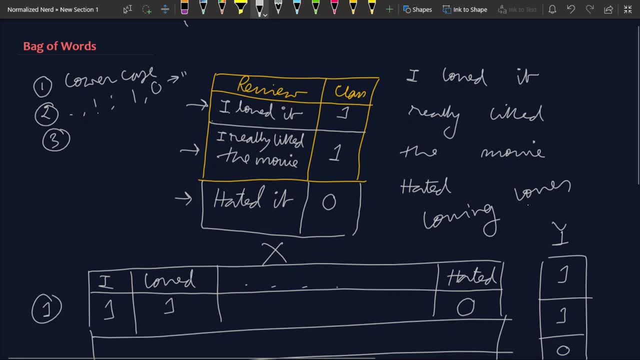 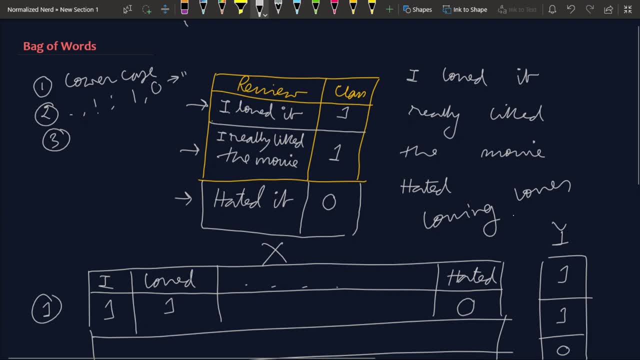 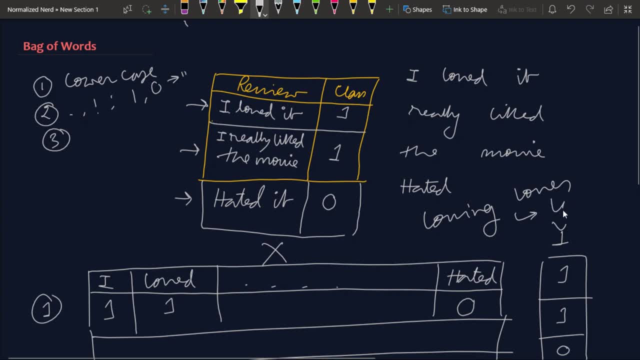 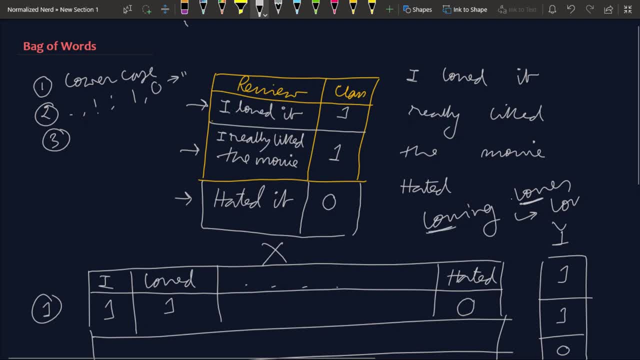 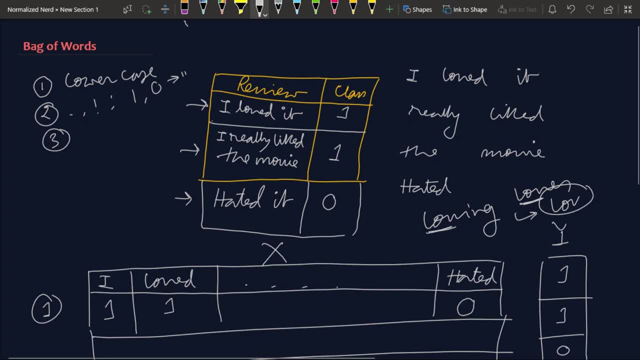 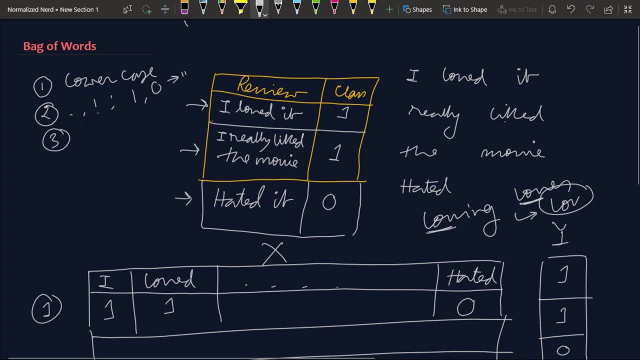 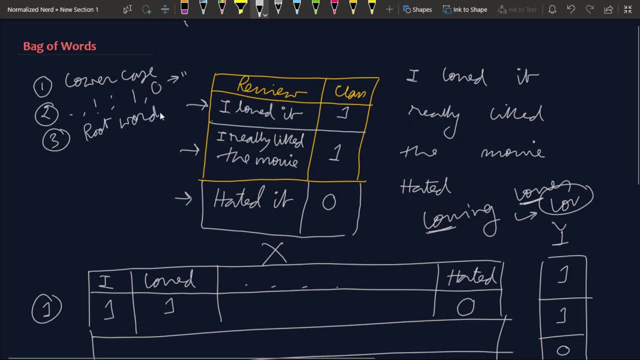 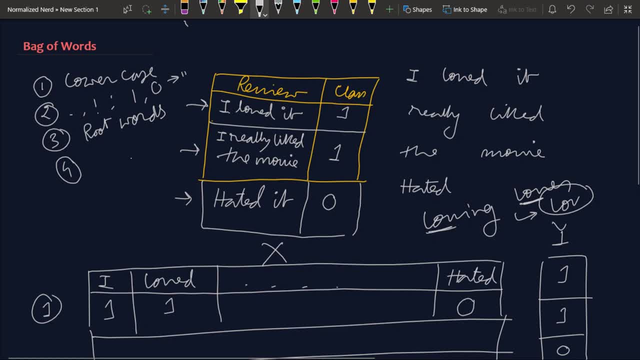 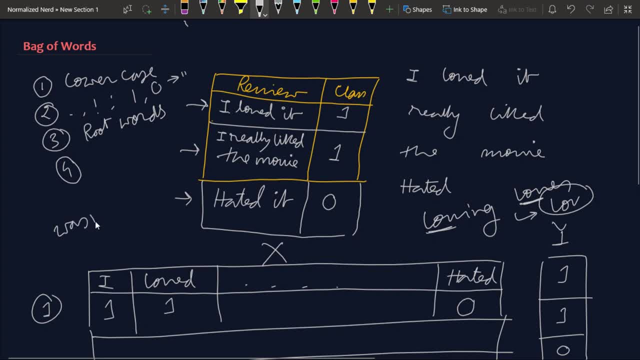 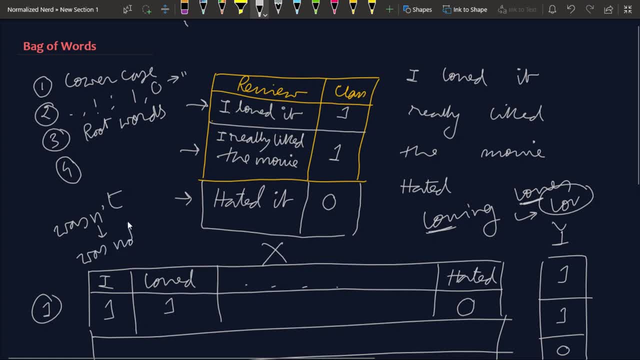 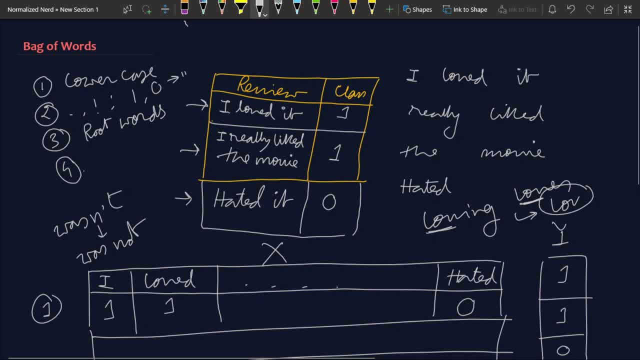 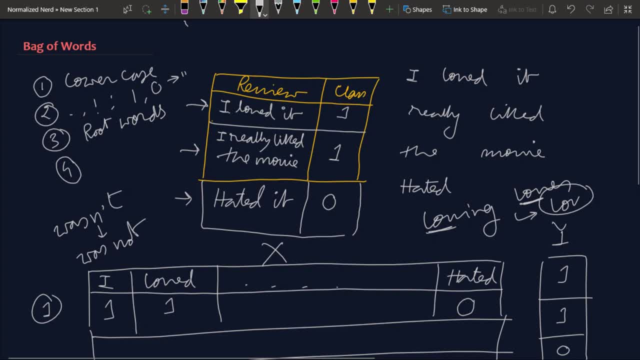 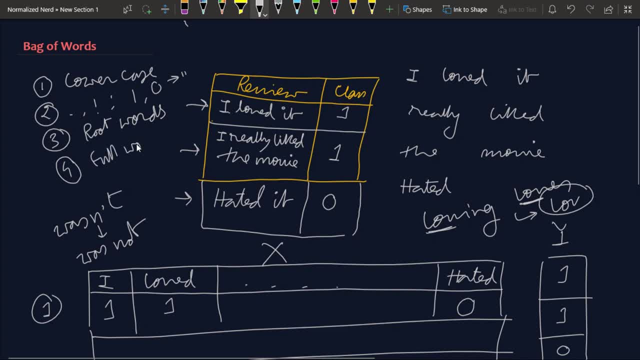 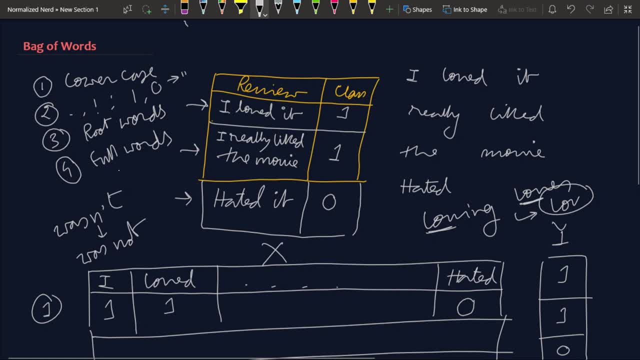 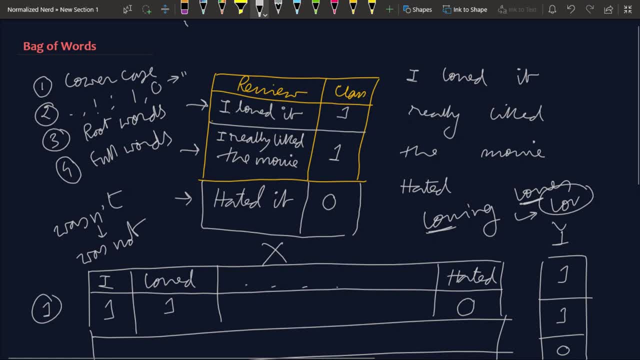 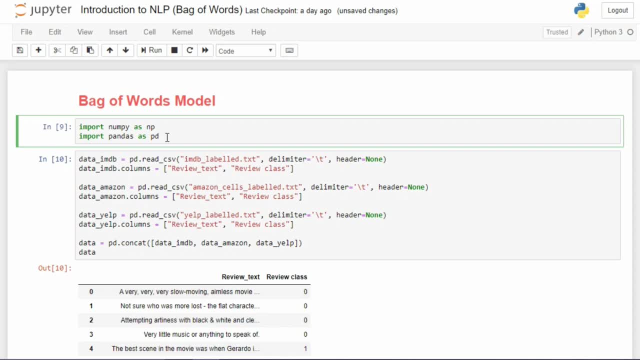 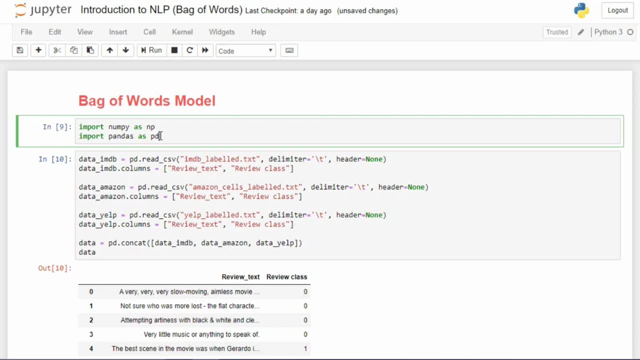 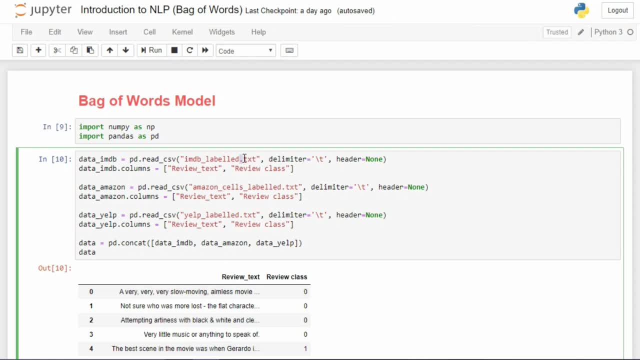 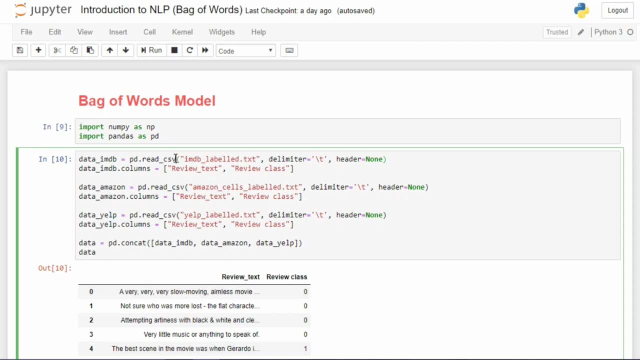 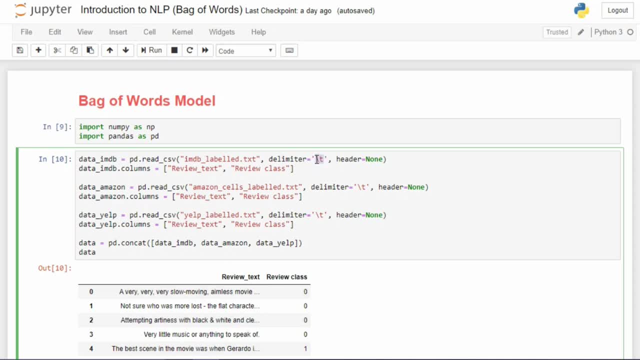 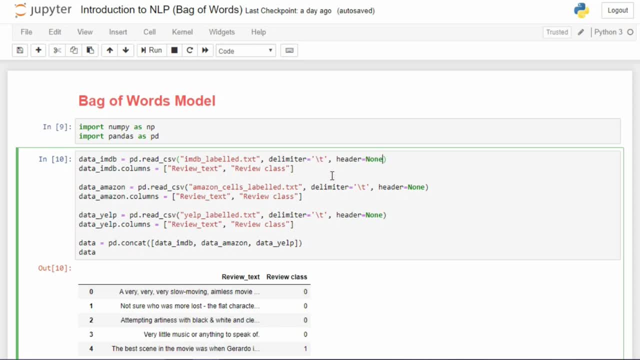 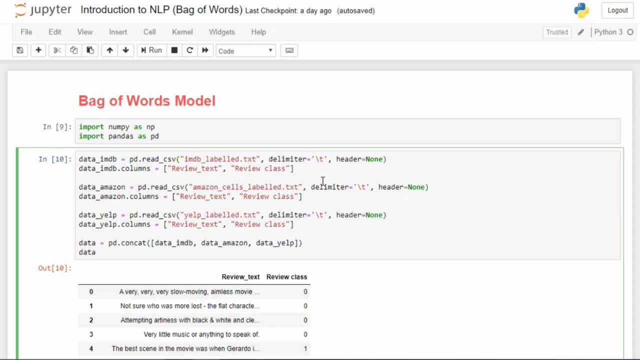 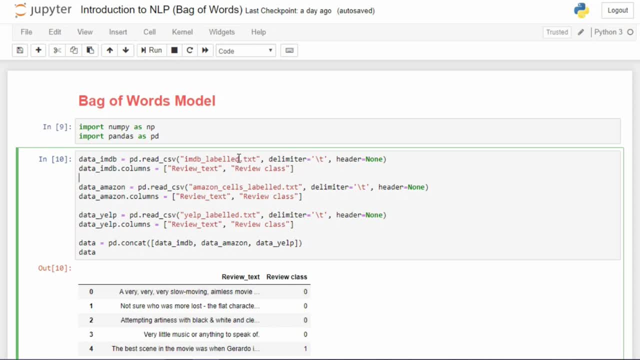 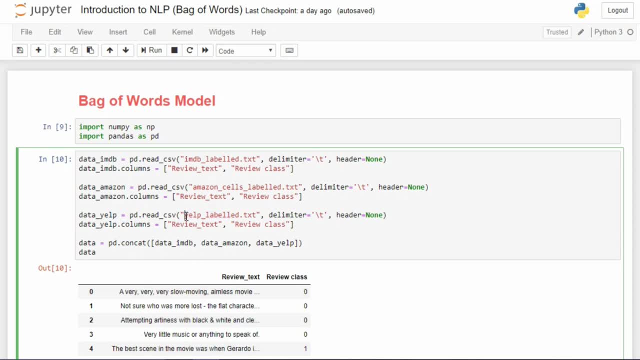 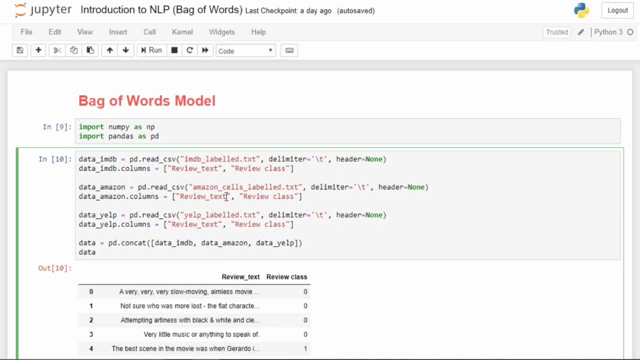 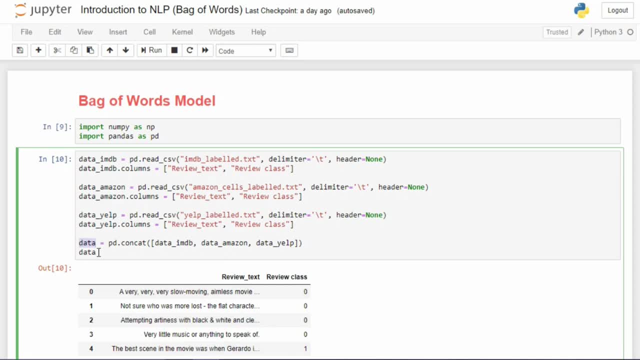 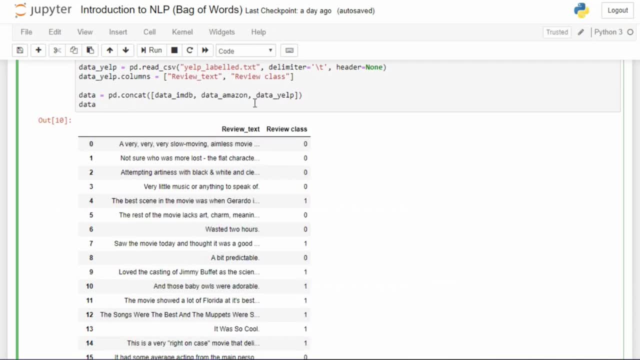 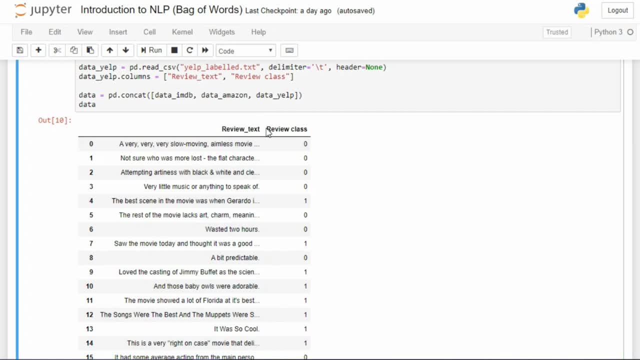 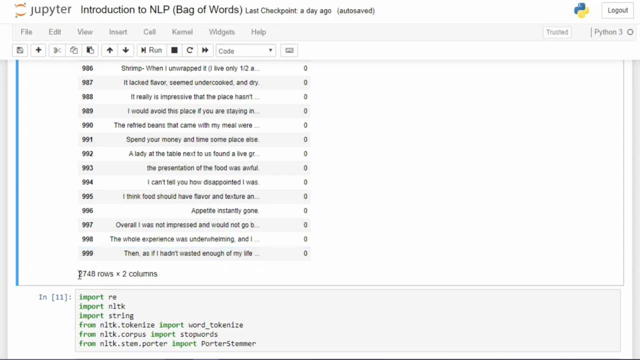 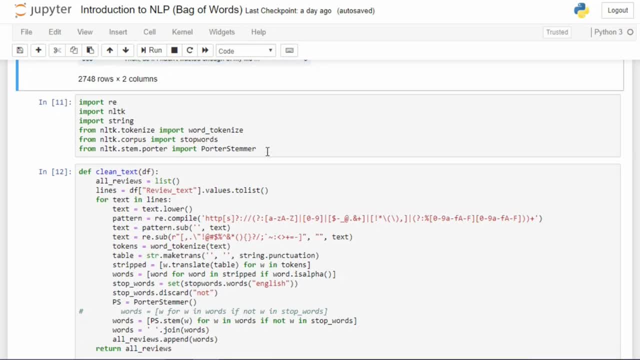 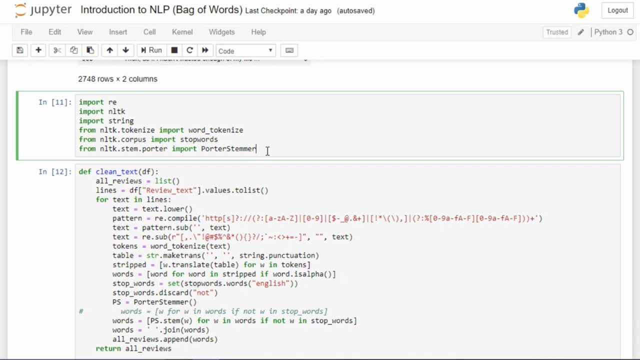 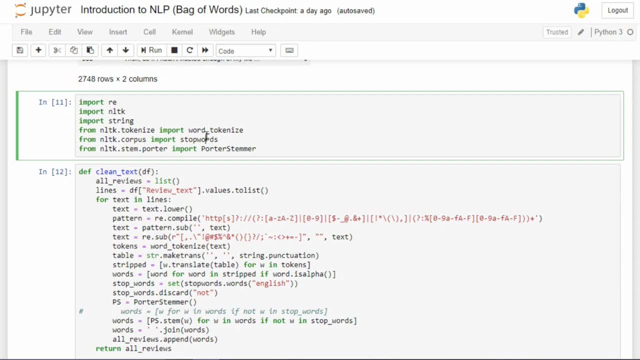 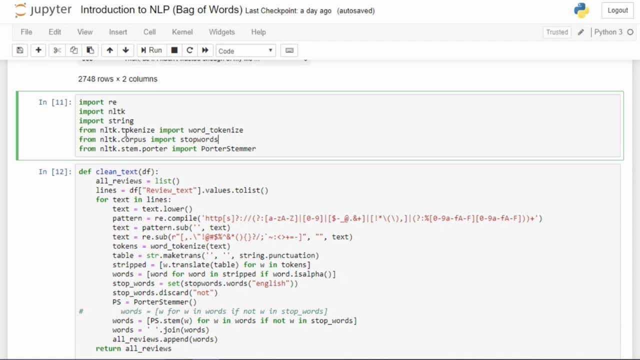 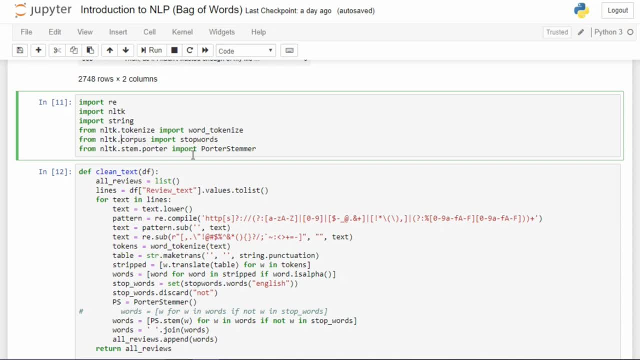 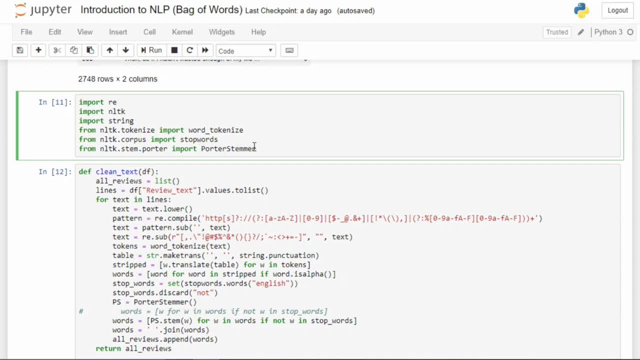 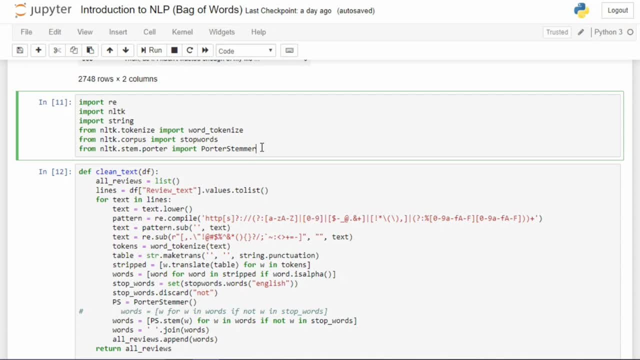 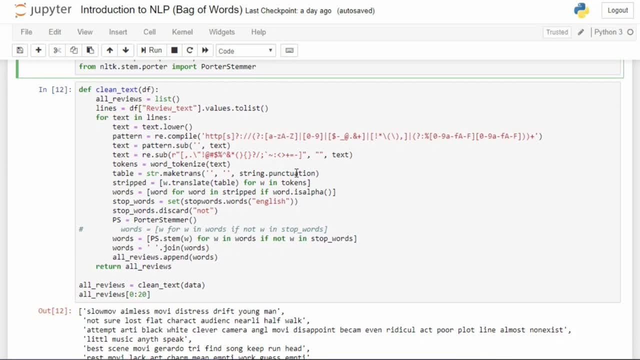 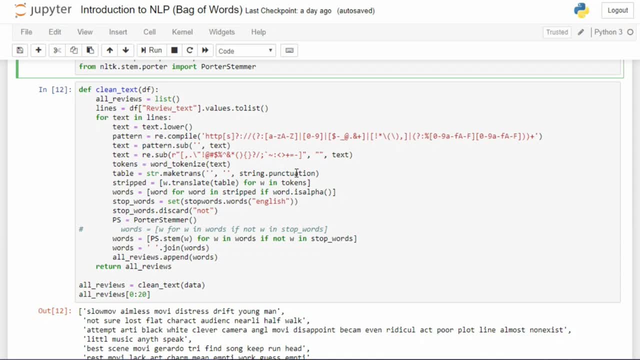 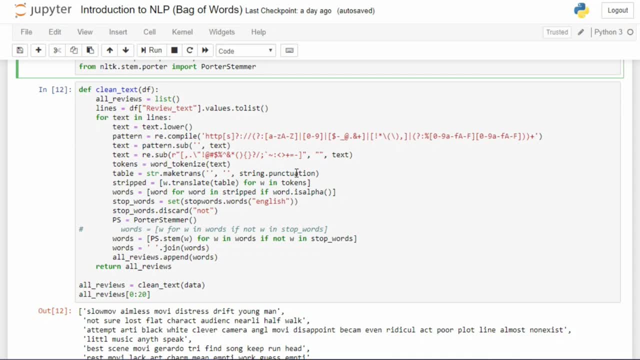 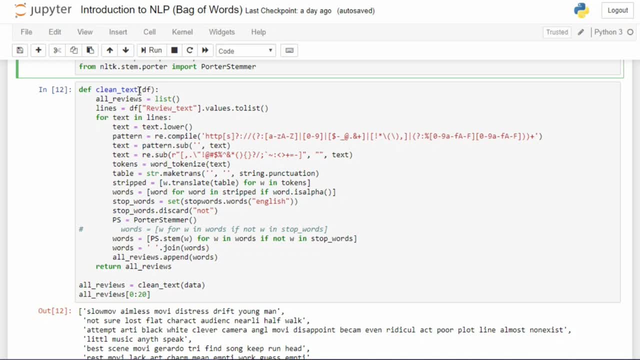 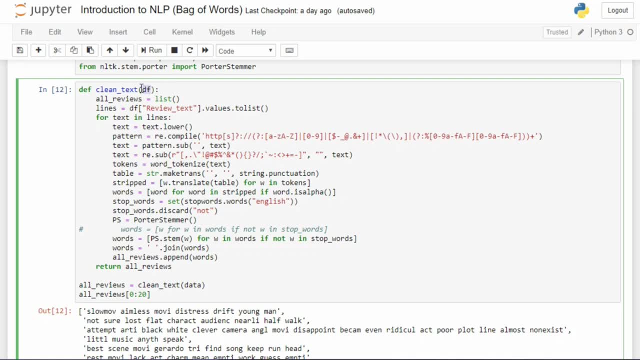 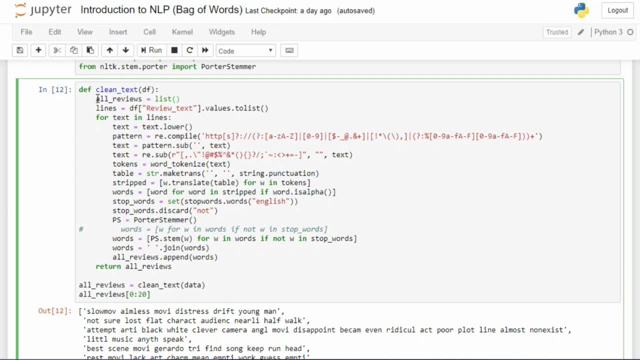 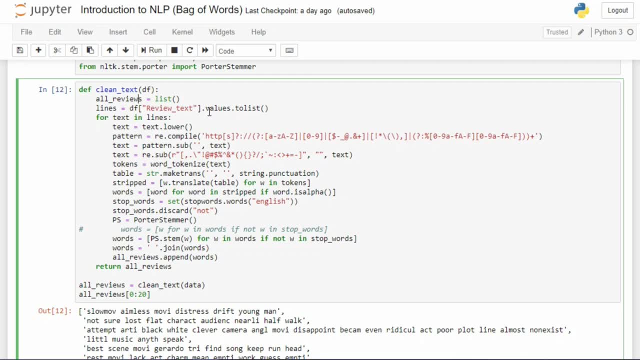 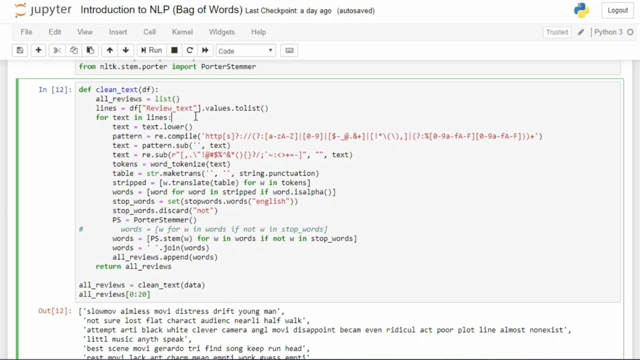 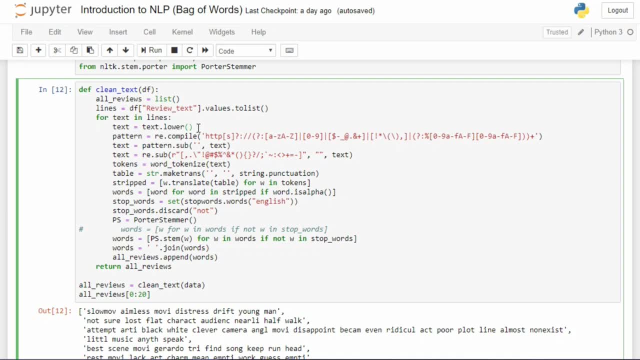 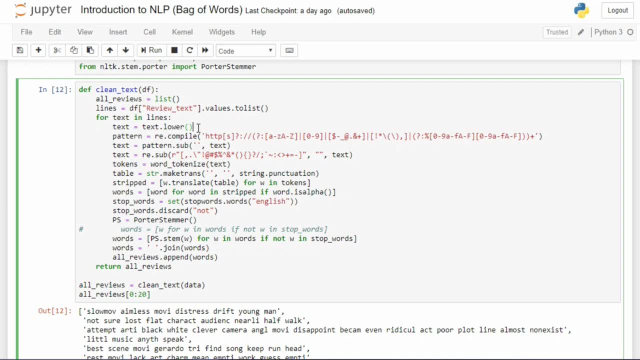 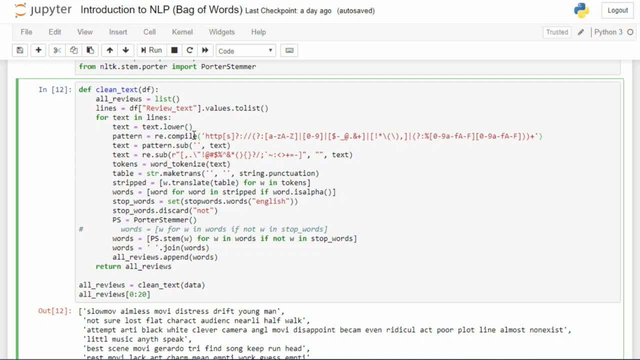 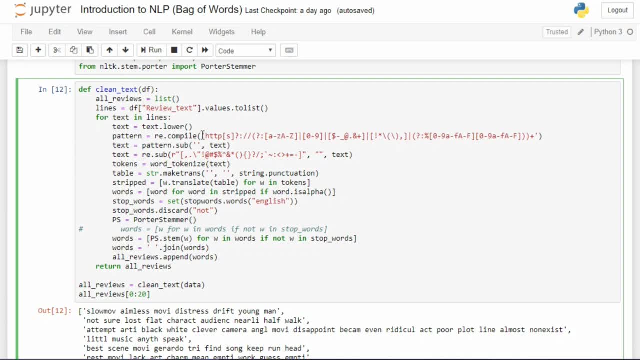 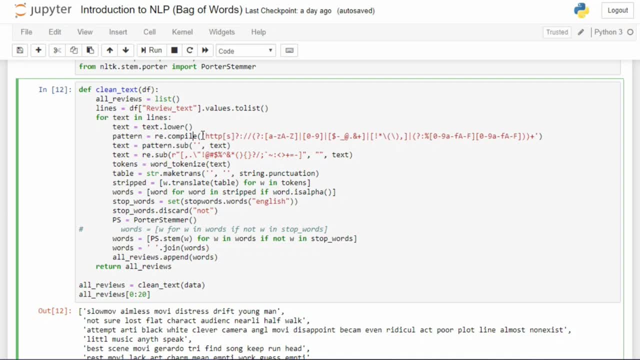 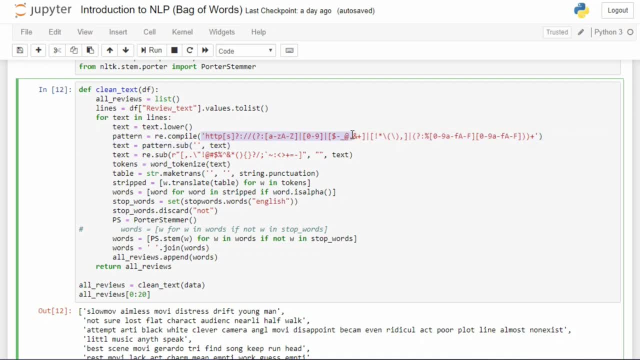 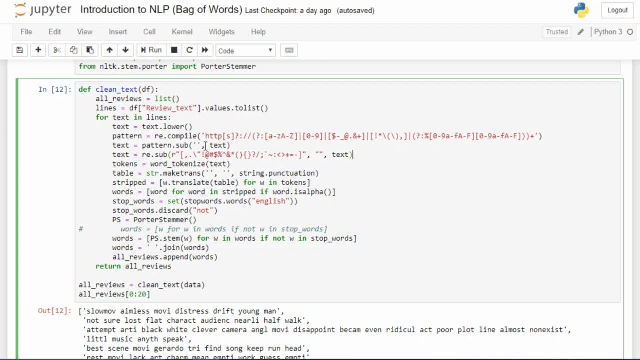 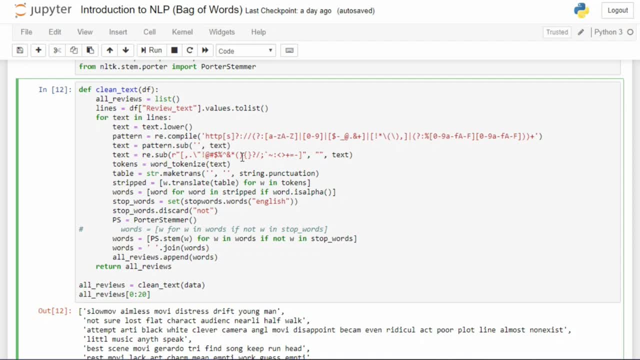 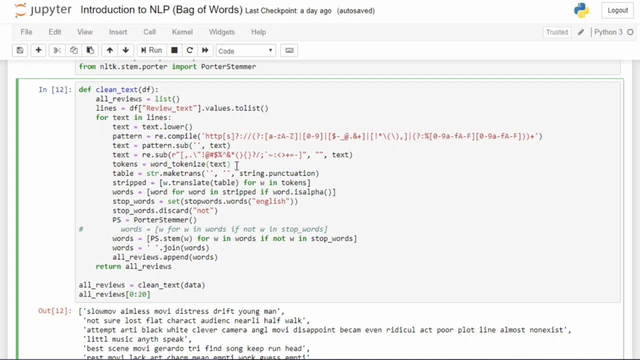 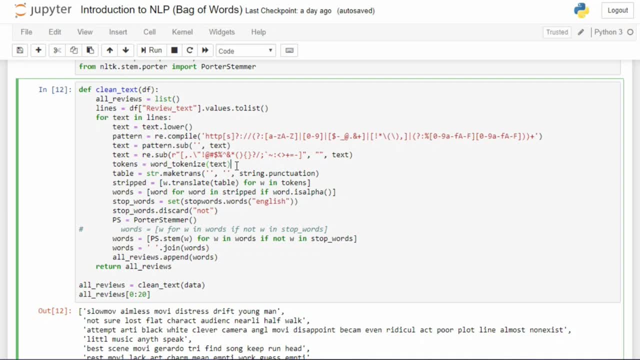 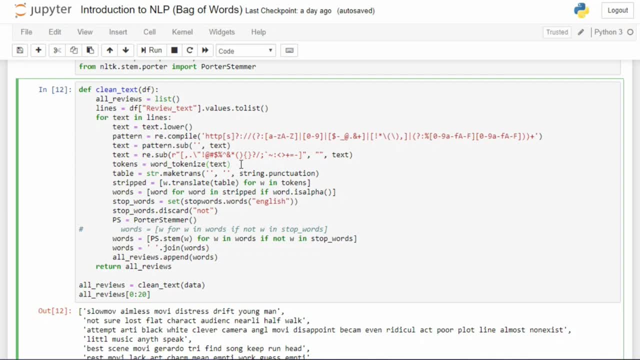 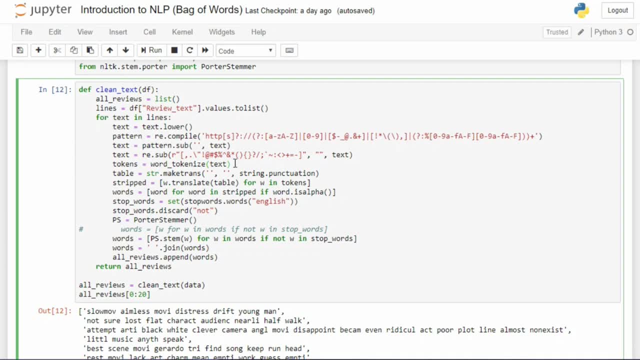 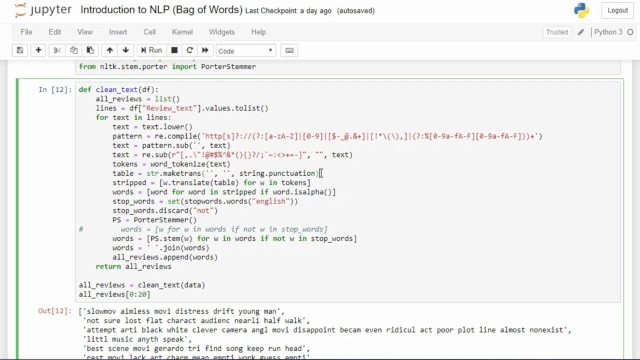 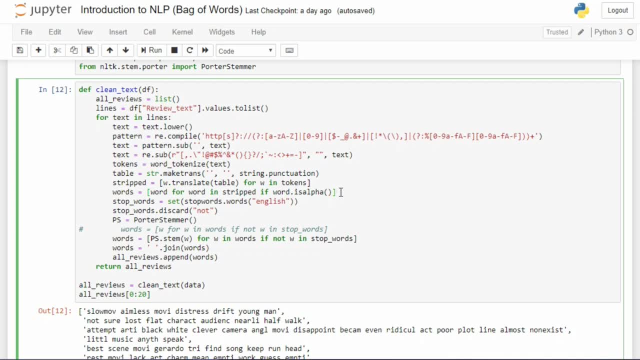 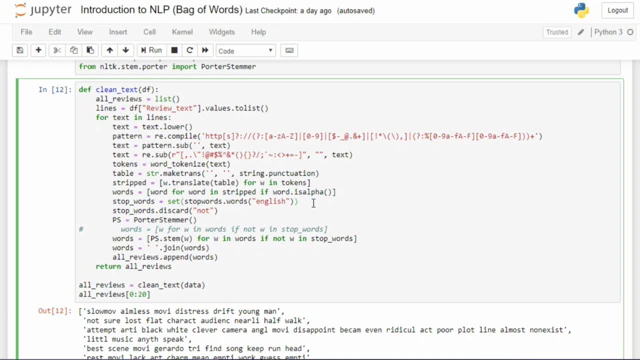 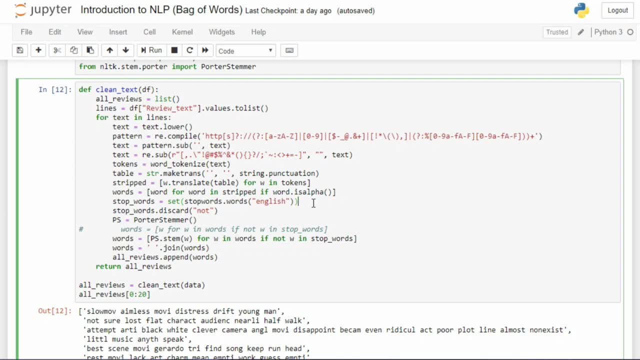 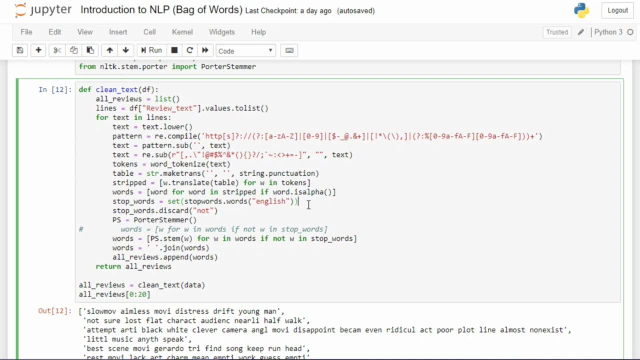 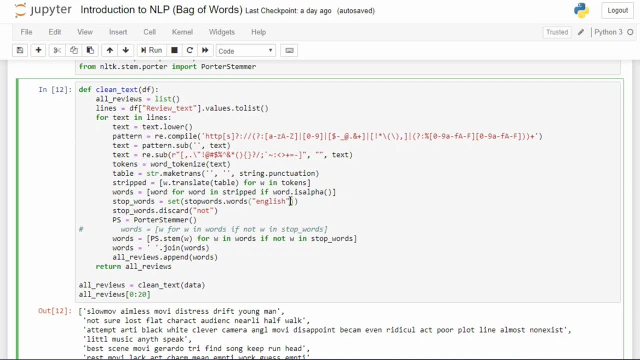 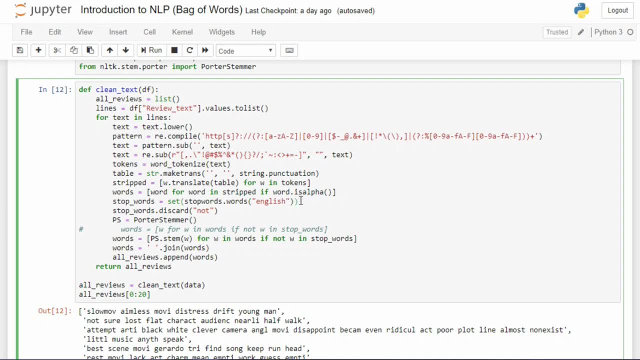 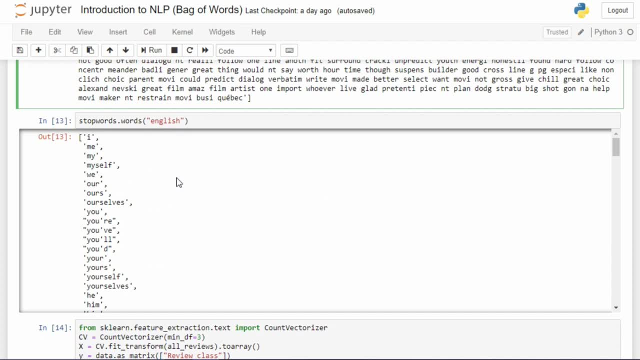 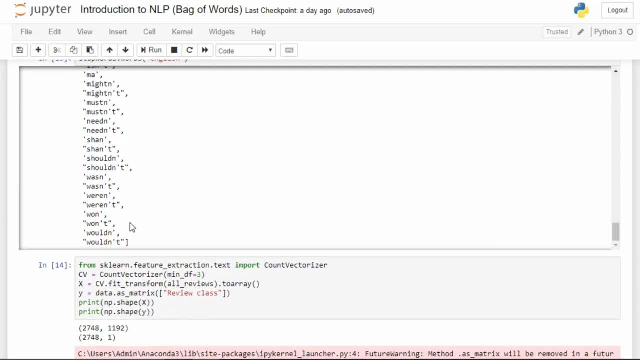 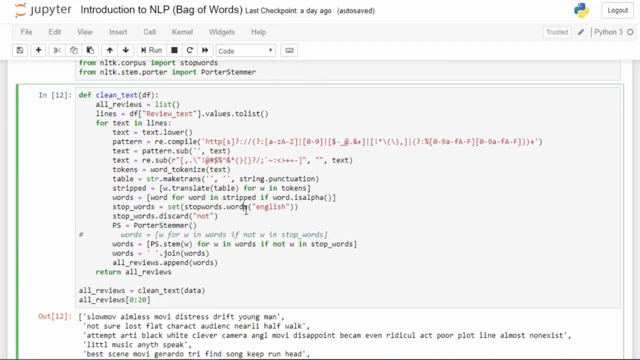 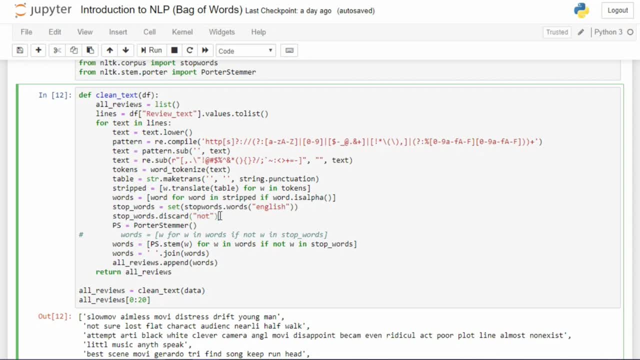 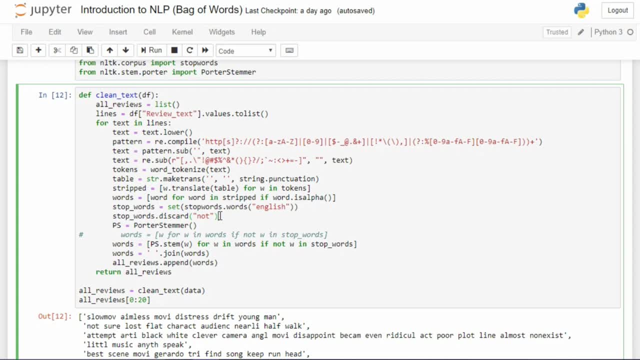 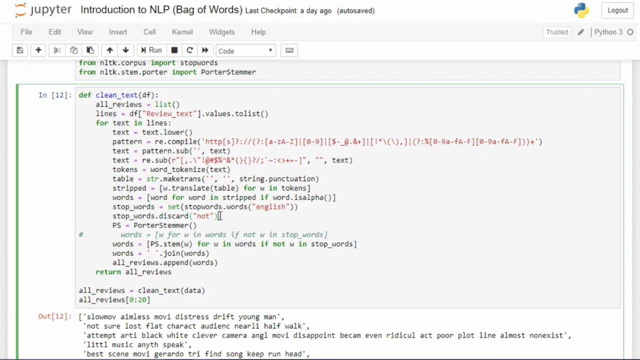 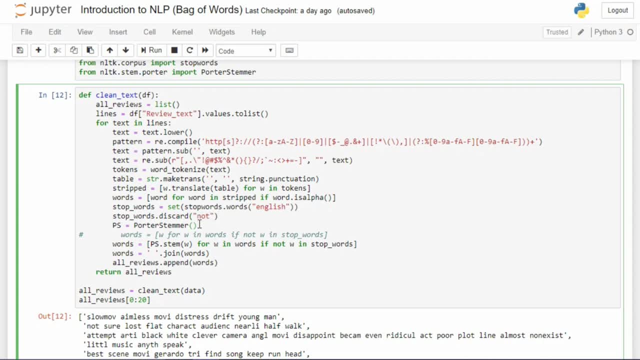 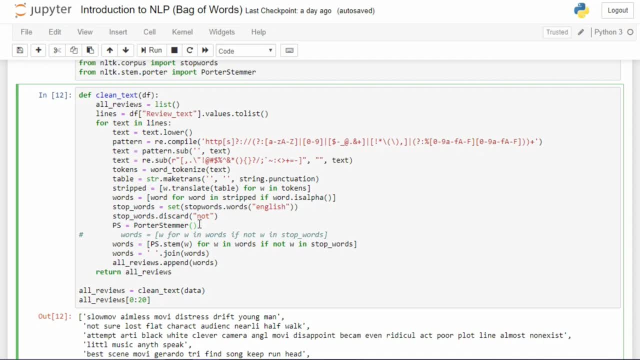 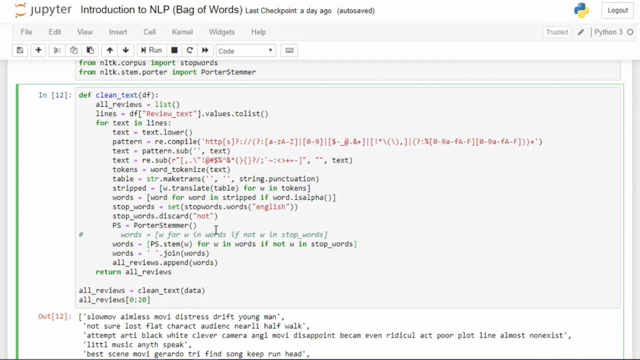 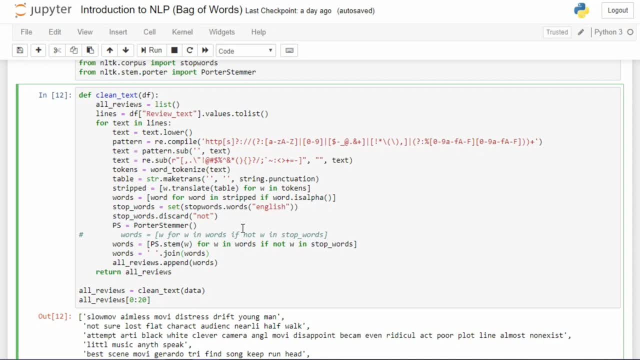 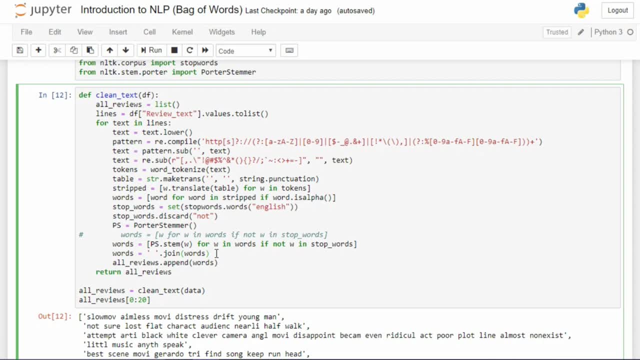 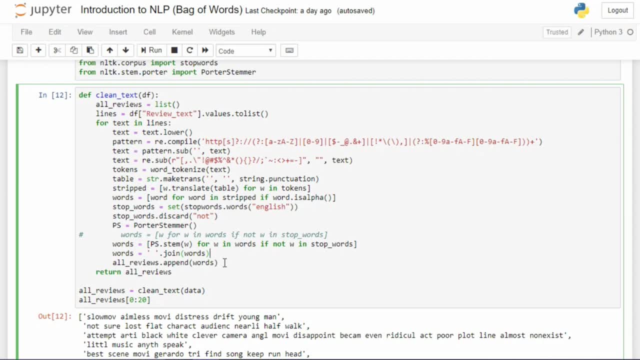 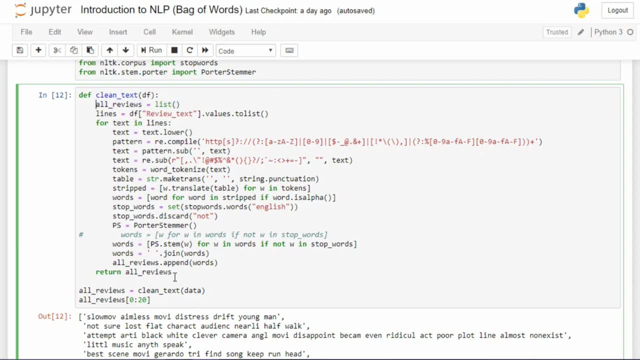 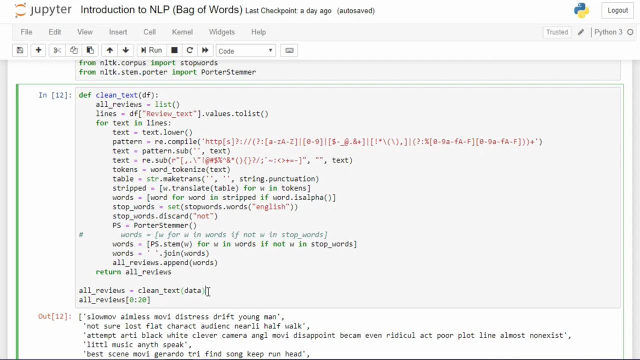 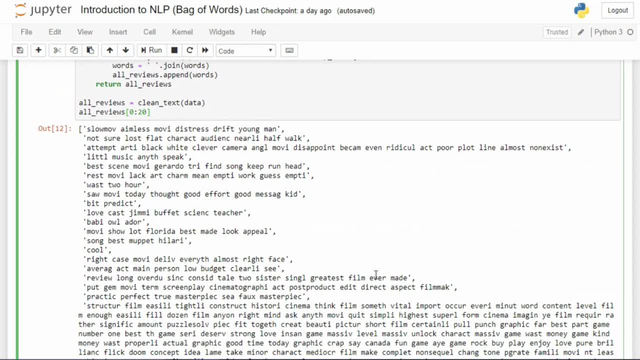 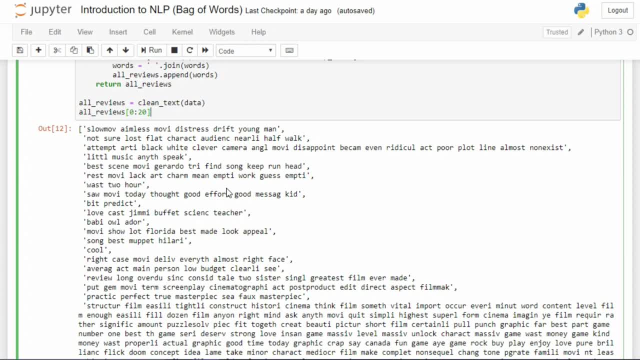 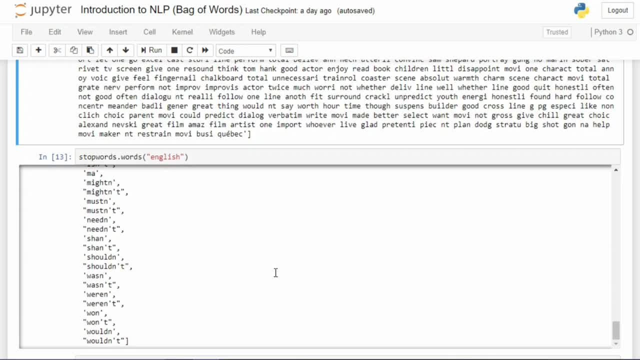 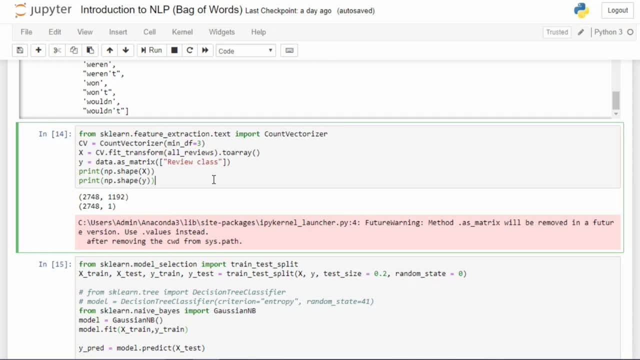 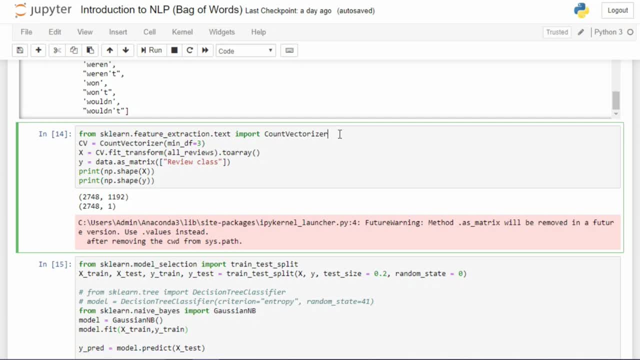 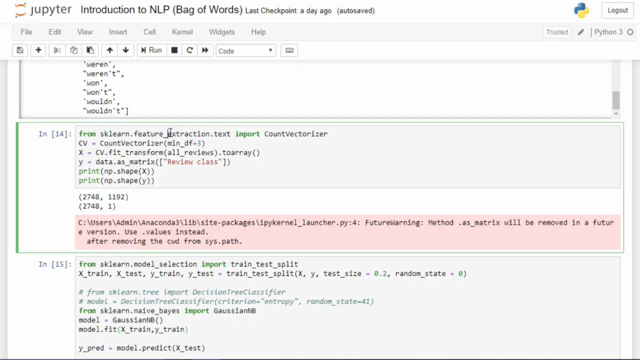 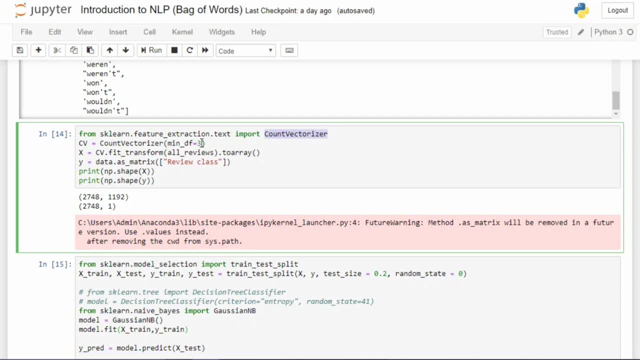 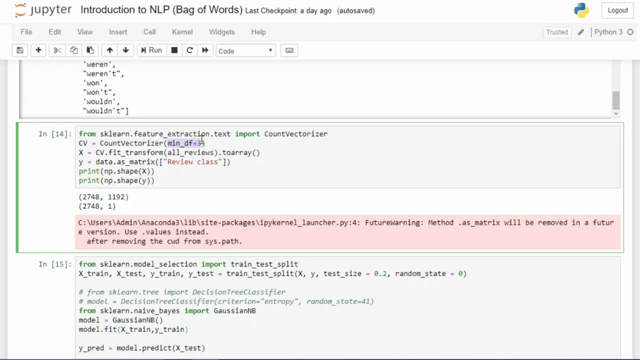 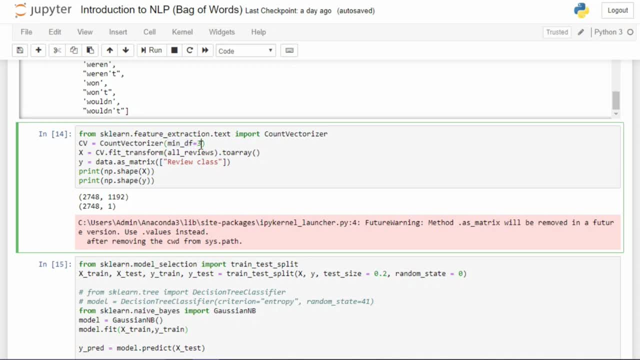 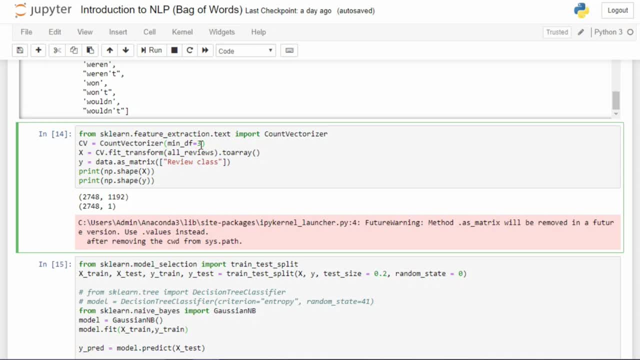 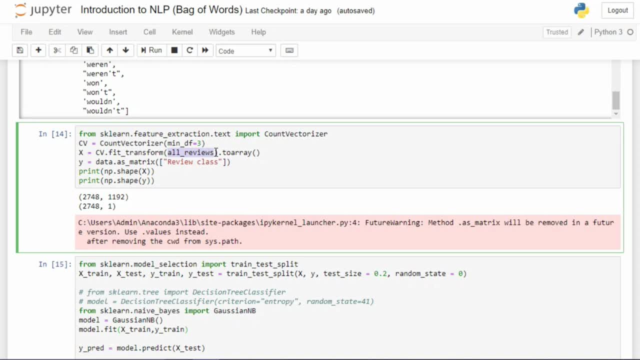 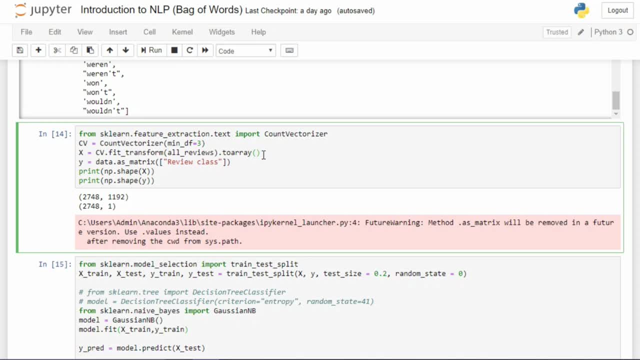 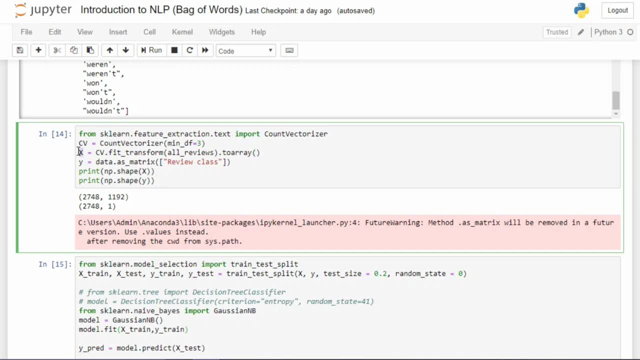 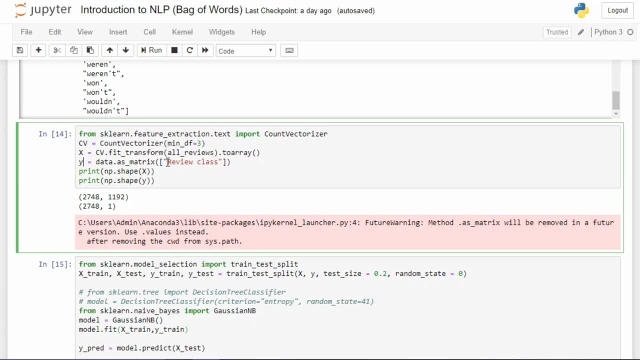 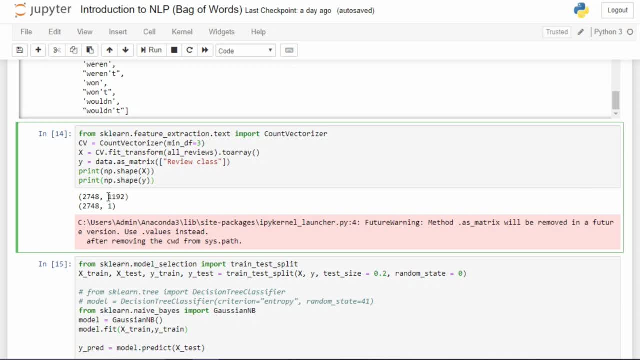 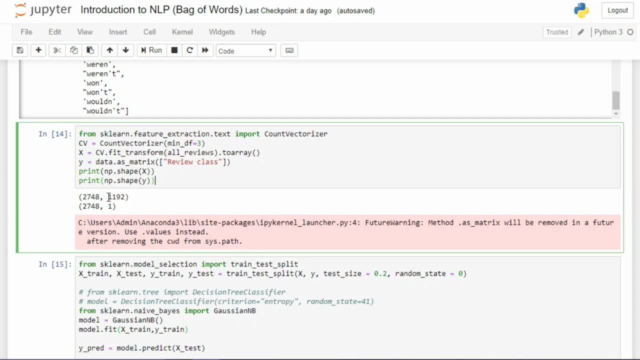 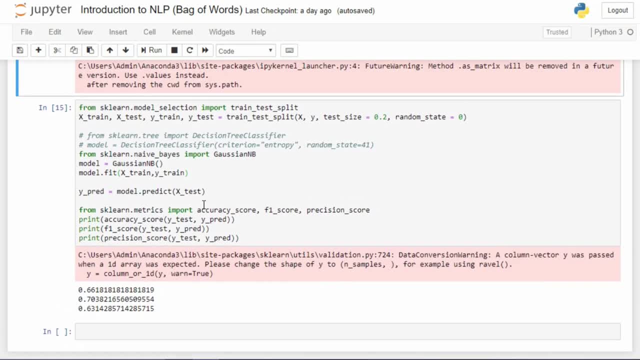 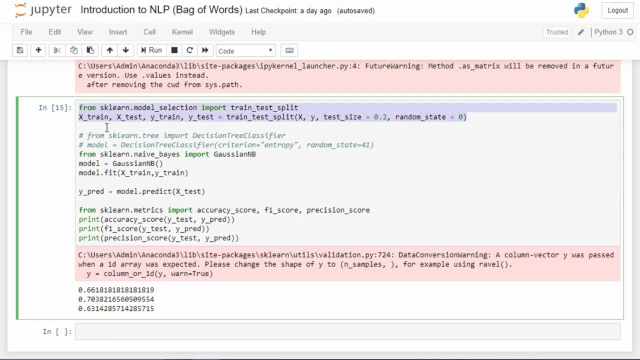 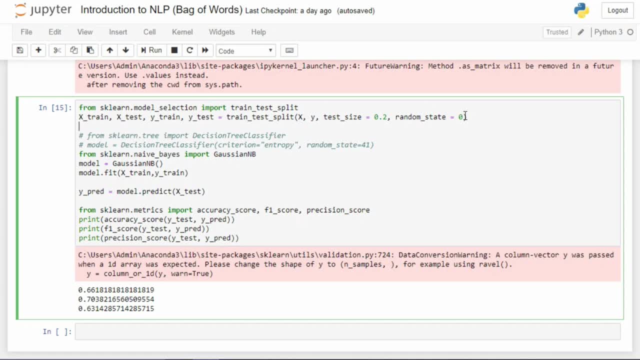 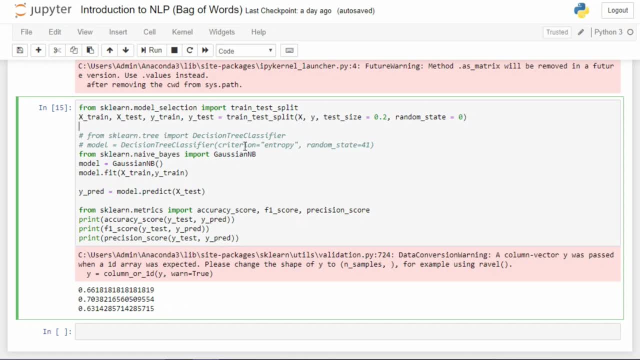 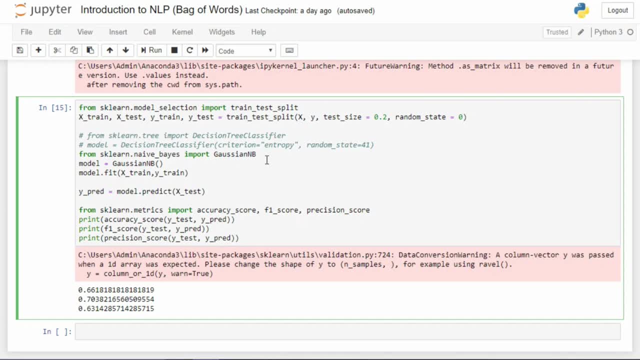 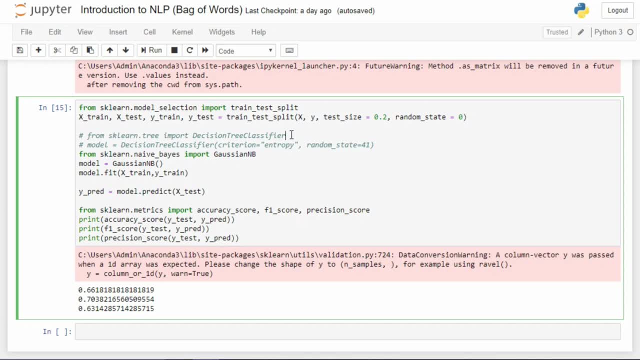 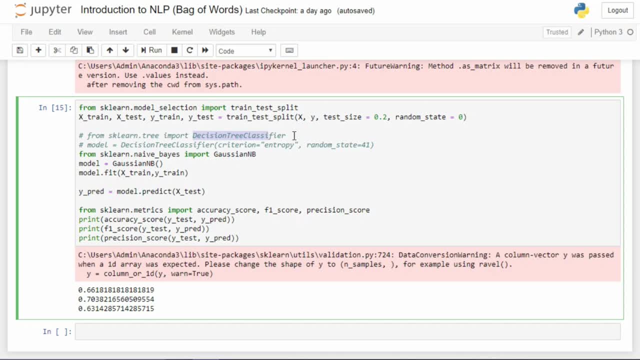 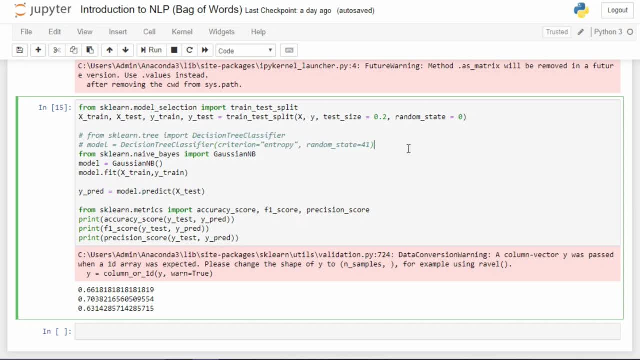 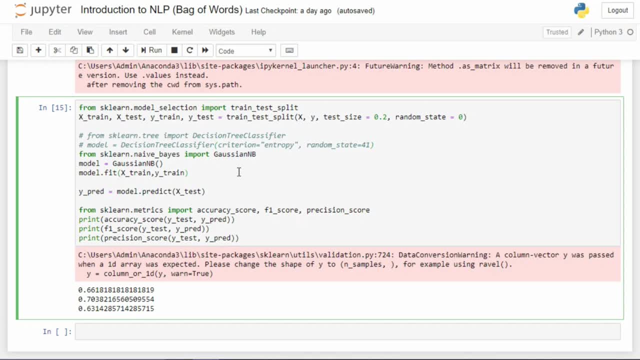 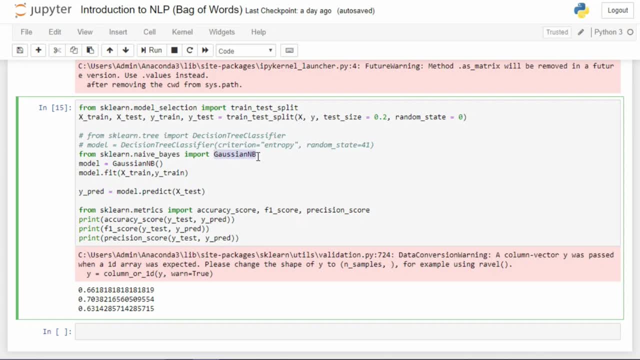 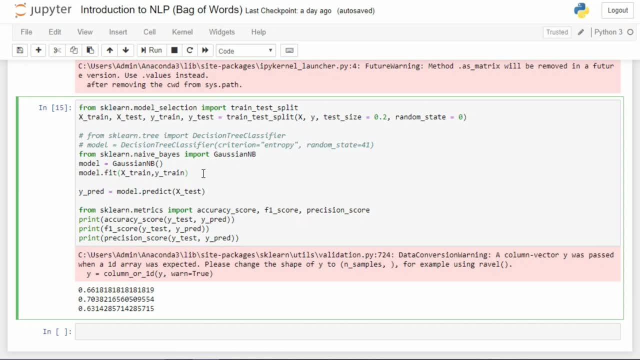 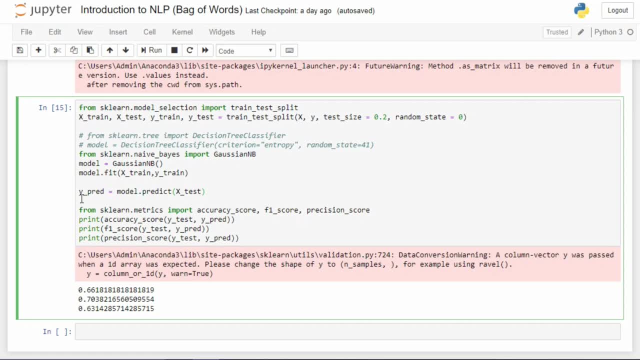 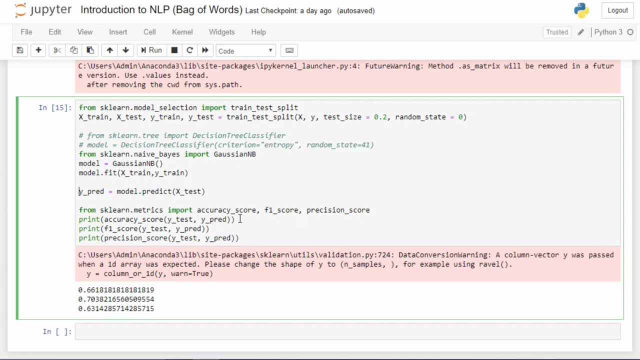 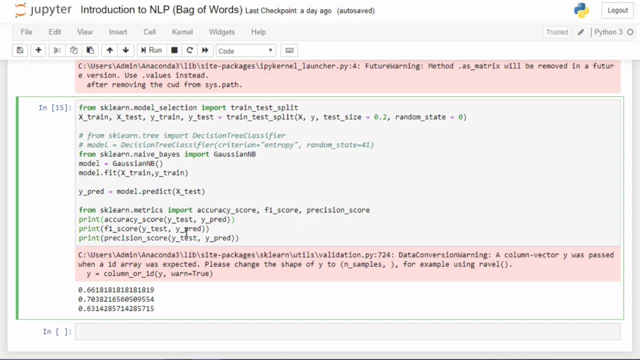 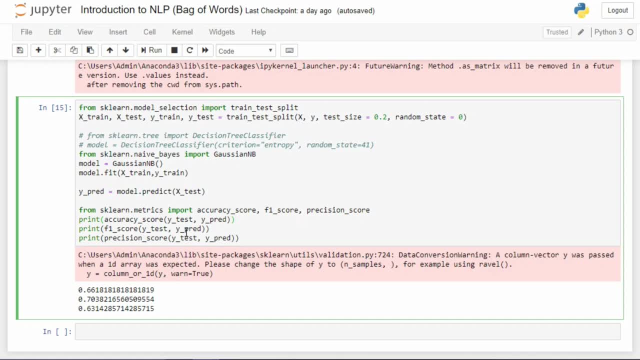 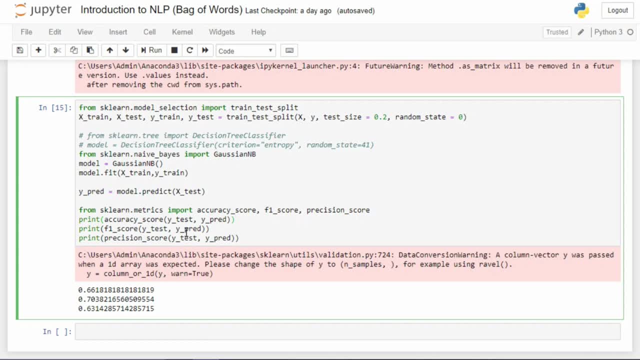 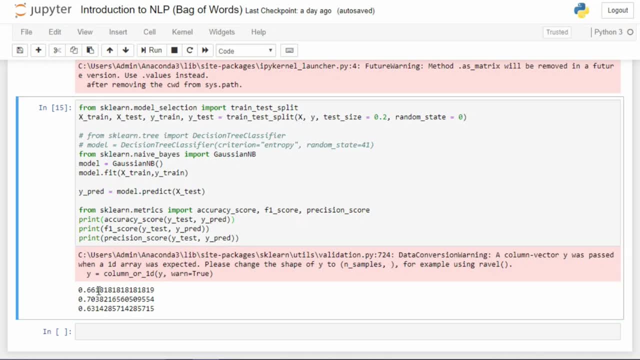 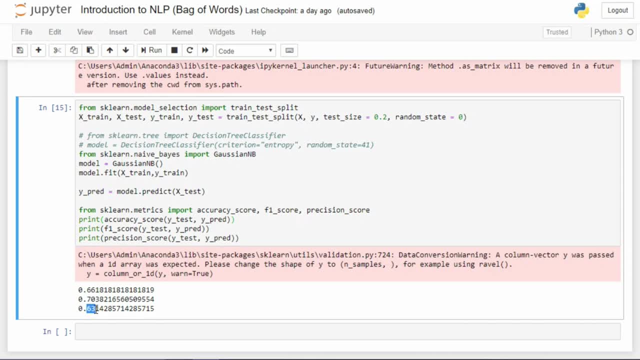 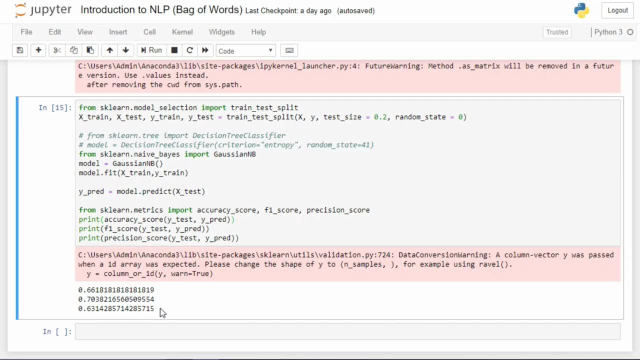 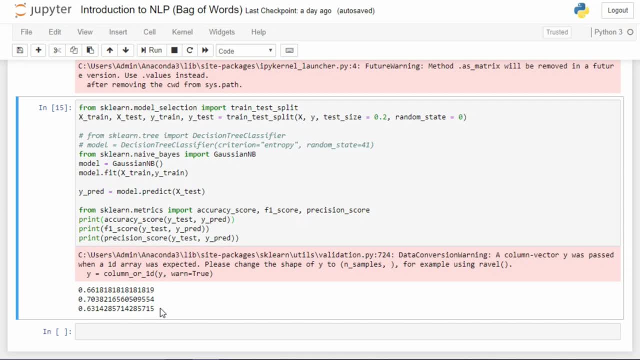 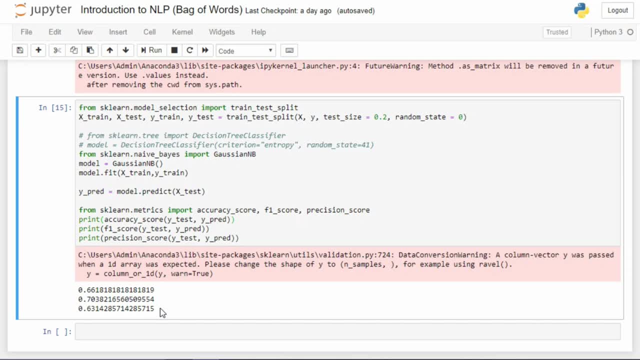 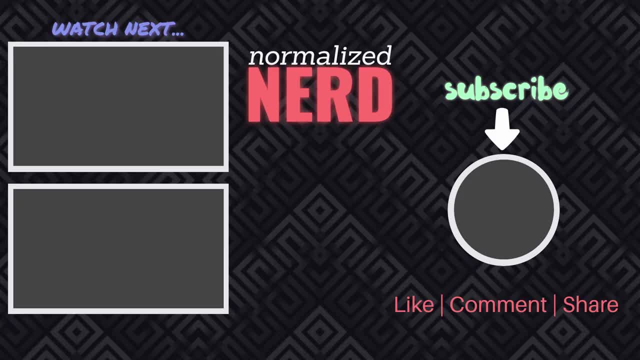 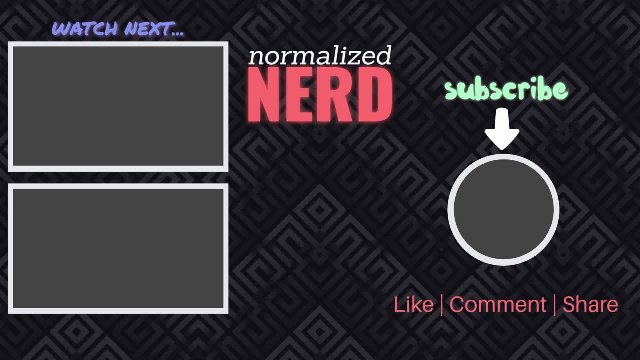 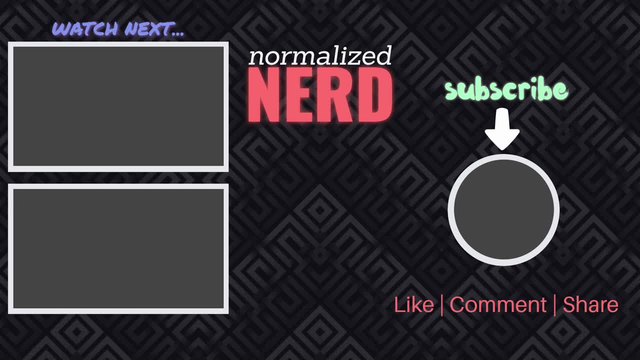 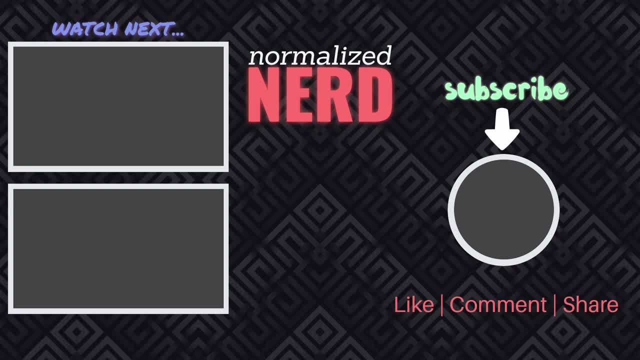